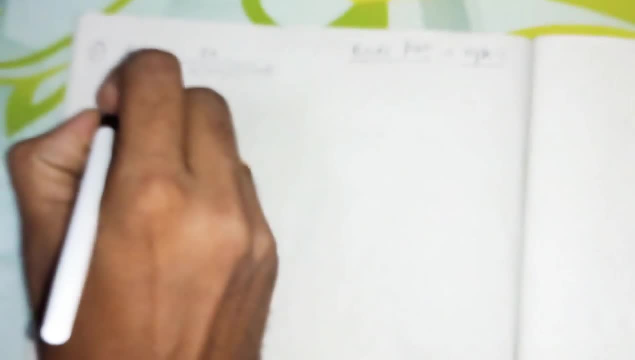 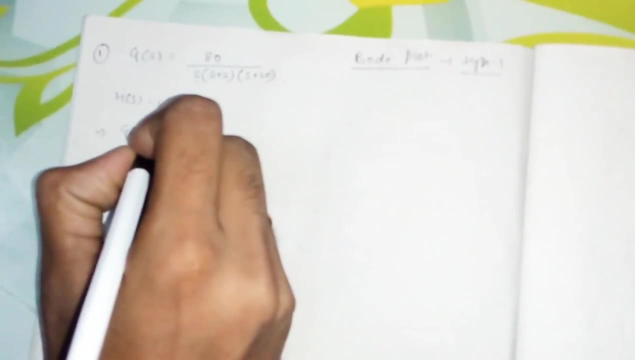 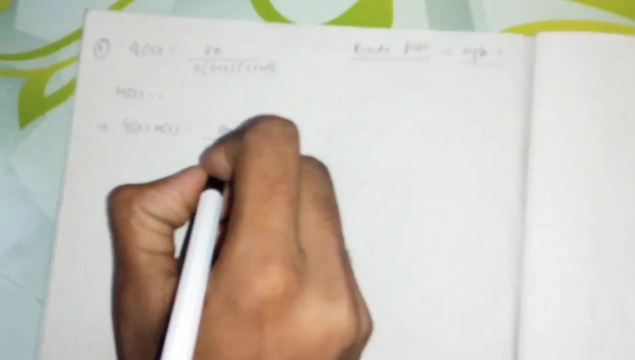 So unity feedback: Hs is equal to 1.. So we will write in the form of Bode, like we will write in the form G of S into H of S is equal to 80 divided by S into S plus 2, S plus 20.. 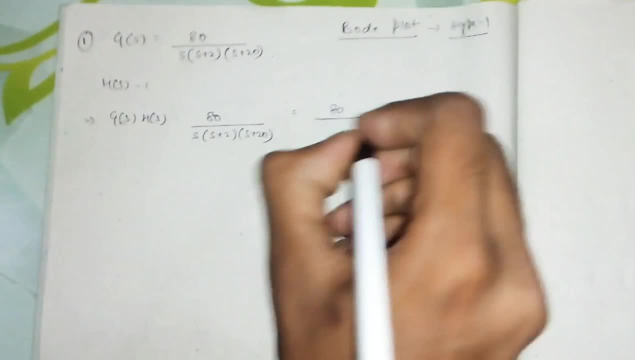 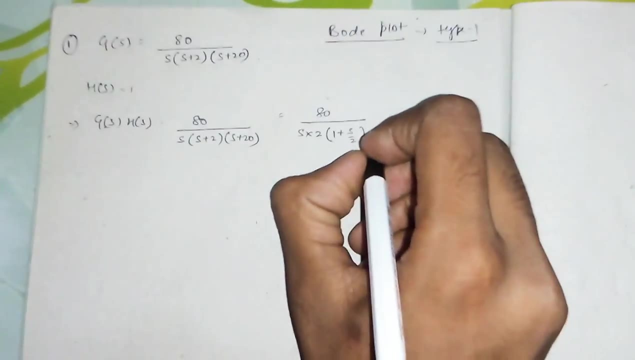 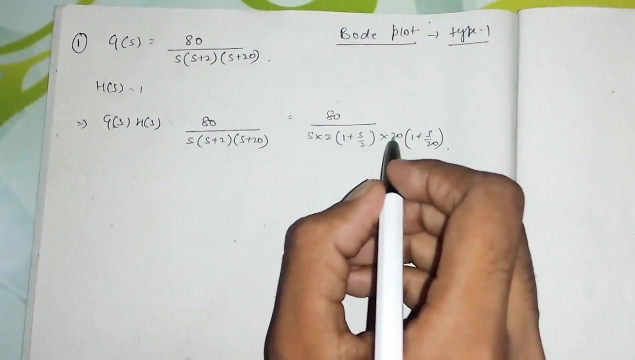 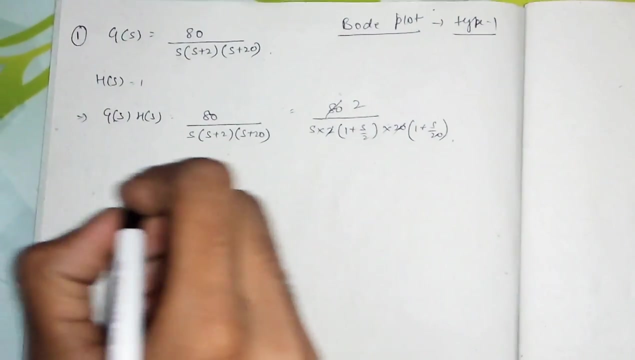 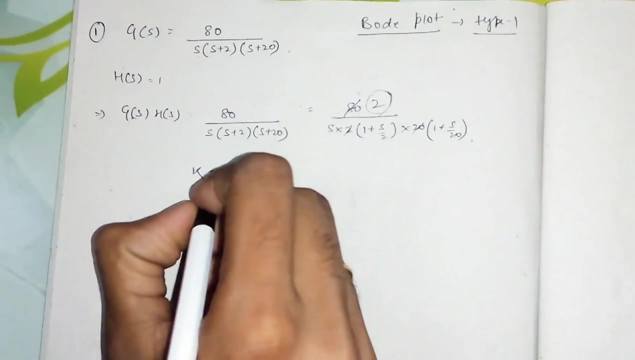 We will write in that form. So S into will take 2 out, 1 plus S by 2.. 20 into 20 will take out 1 plus S by 20.. We will simplify it. That is 20 into 2.. 4 like 40 into 2.. So this part which is there that is known as K, That is a K. K is equal to 2.. 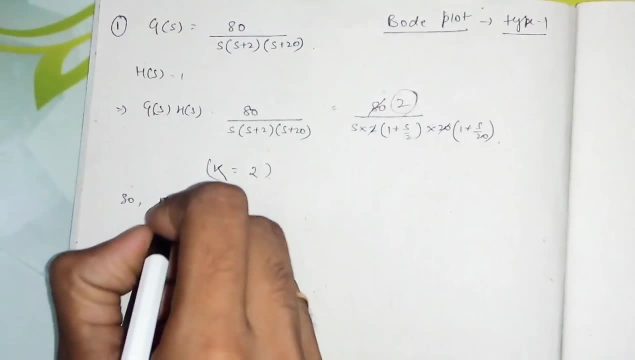 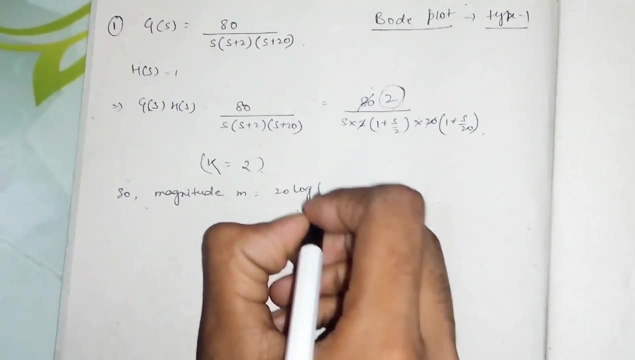 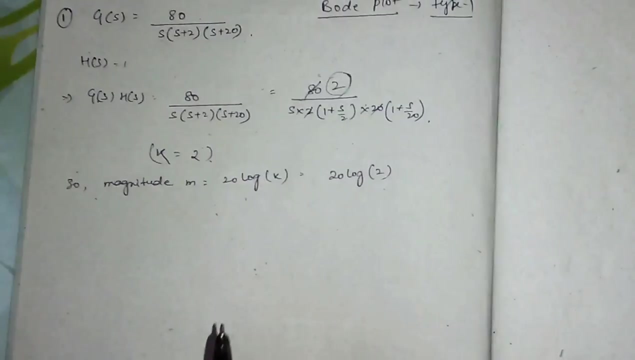 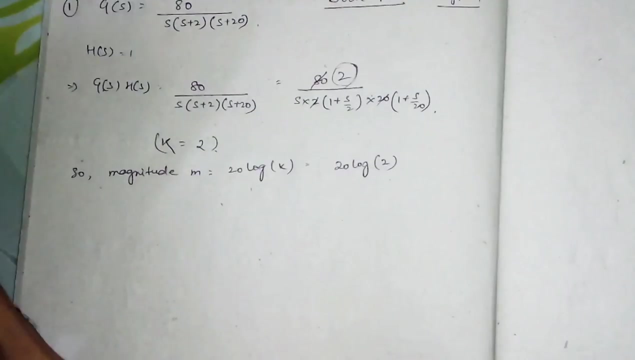 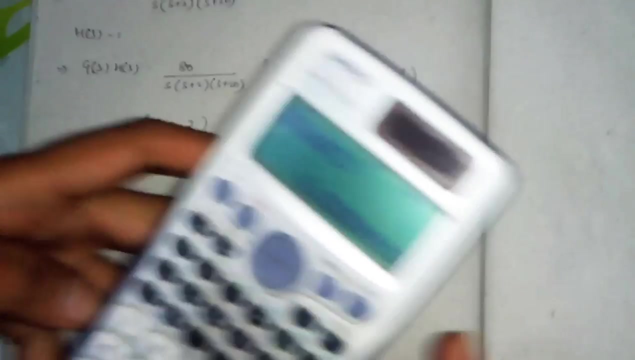 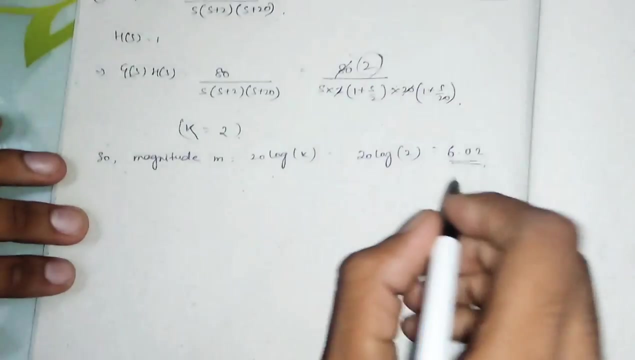 So immediately, we will find out the magnitude. Magnitude M is equal to 20 log K, So 20 log 2.. We will calculate it. We will calculate it as 20 log 2.. That is 6.02.. This is our magnitude. 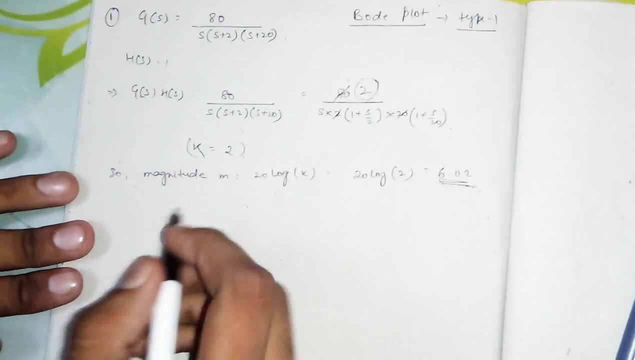 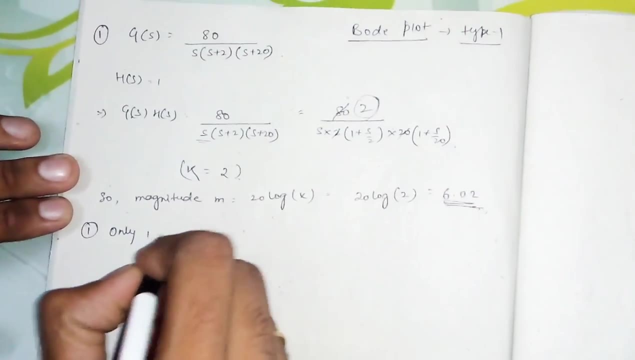 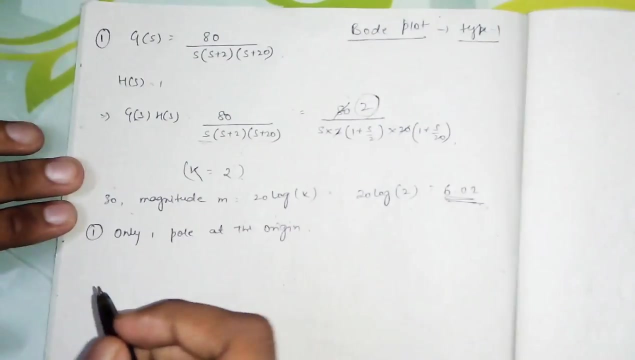 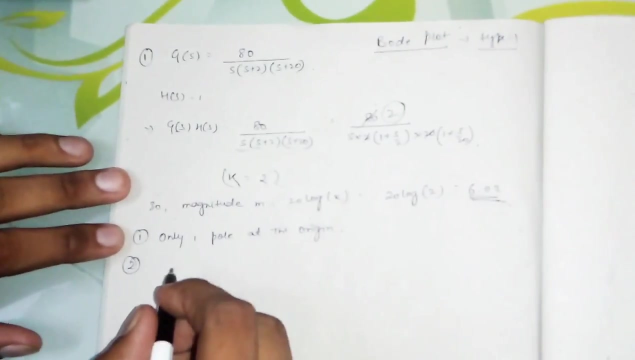 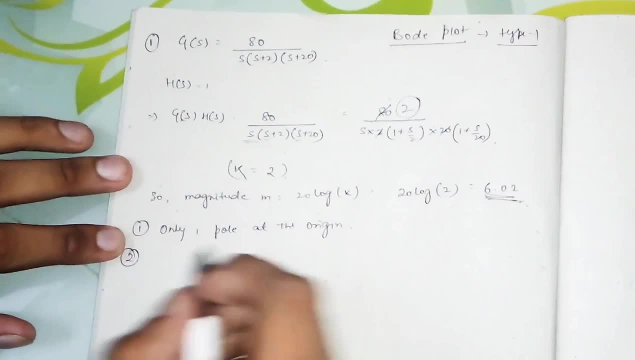 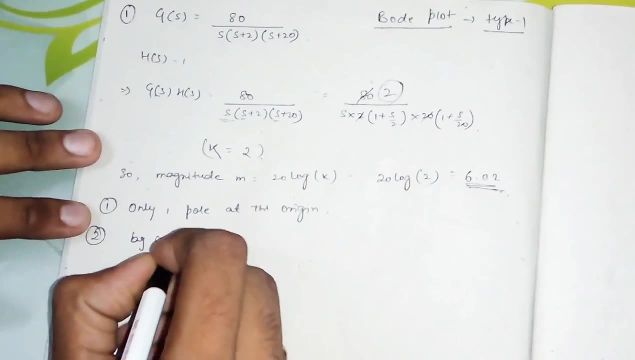 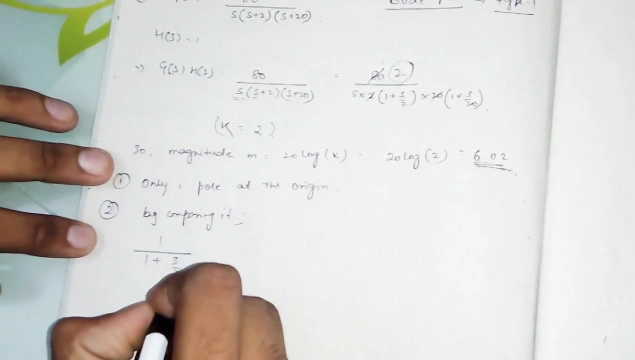 So we will. So we will try to solve it. That is S by 2 and S by 20.. So we will compare By comparing it: 1 divided by 1 plus S by 2.. That is, we can write that T1 is equal to 0.5. 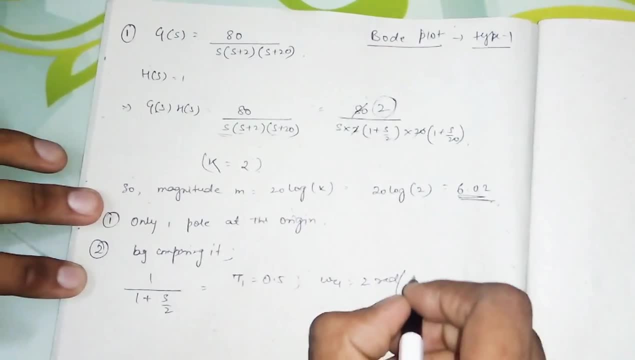 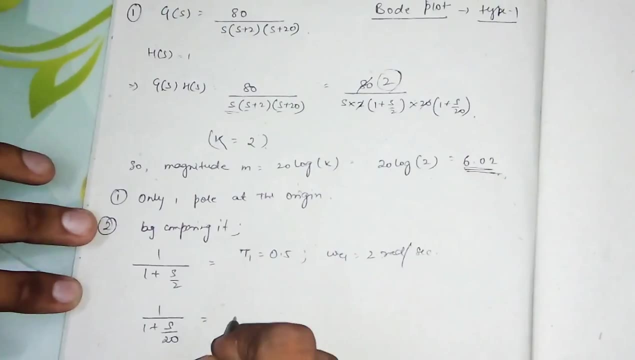 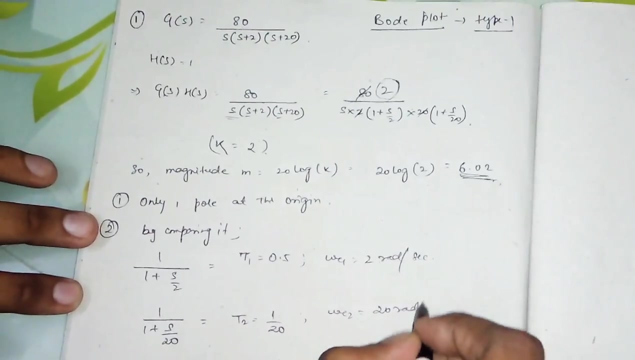 Omega C1 is equal to 2.. The radian is rad per second. Similarly the second one, 1 plus S by 20, that is T2 is equal to 1 by 20, or Omega C2 is equal to 20 rad per second. 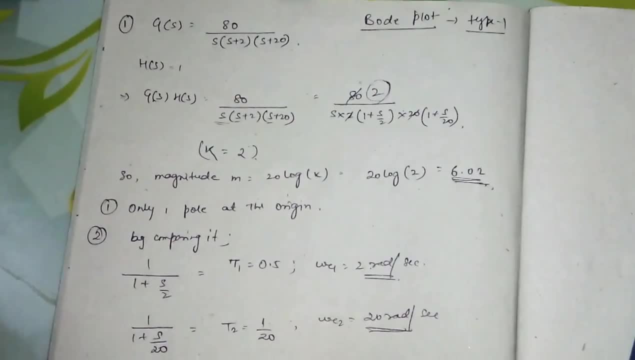 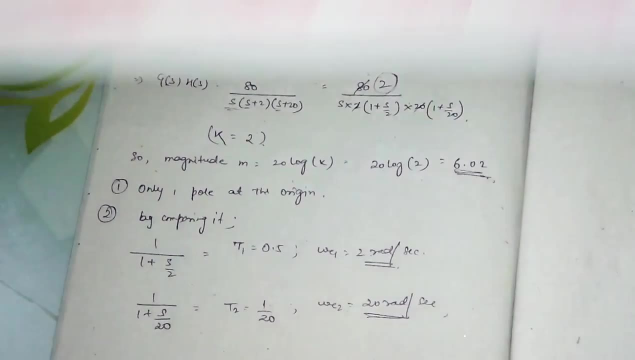 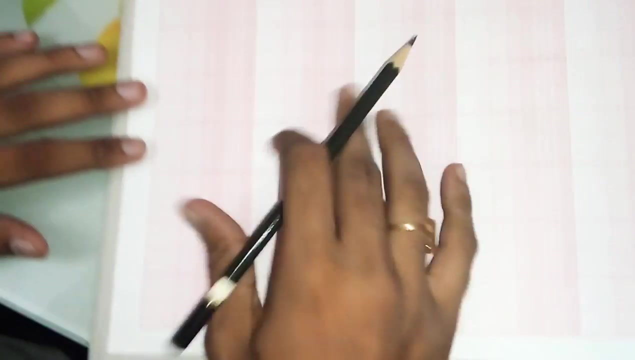 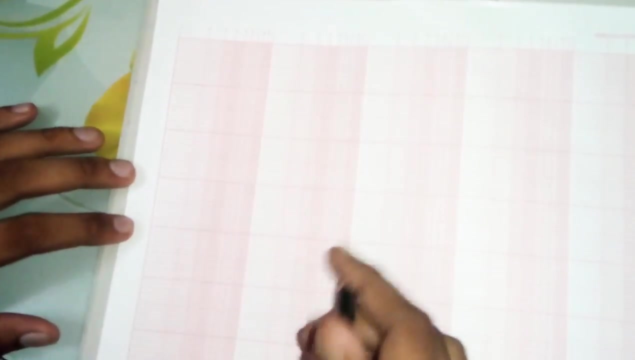 So these are the two Omega values which we have got, and now we will try to plot this magnitude in a graph sheet. This is a graph, This is a logarithmic graph, So we will plot first half as a magnitude and then phase. So phase will come later. 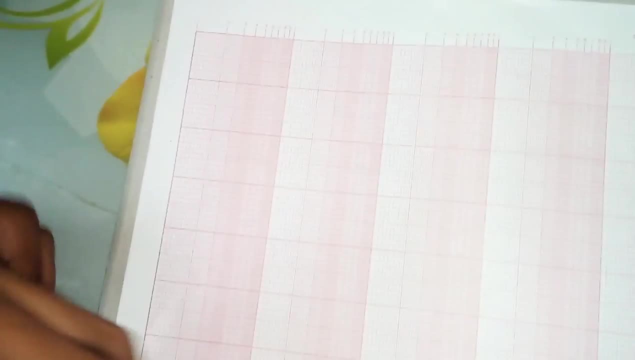 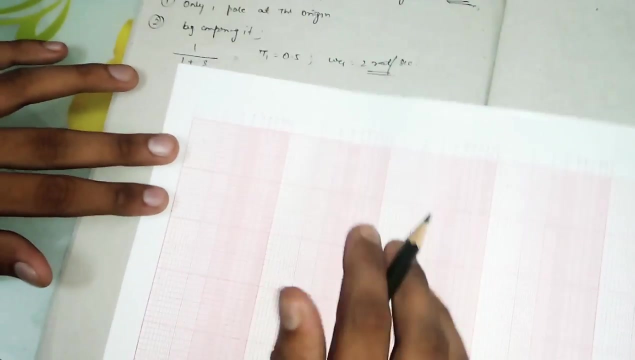 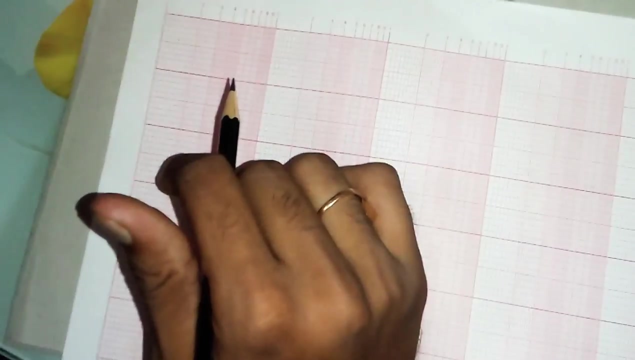 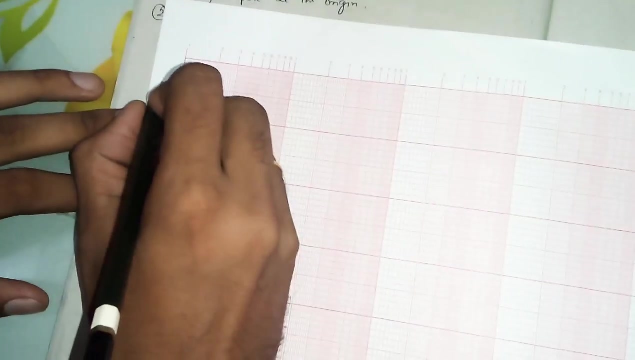 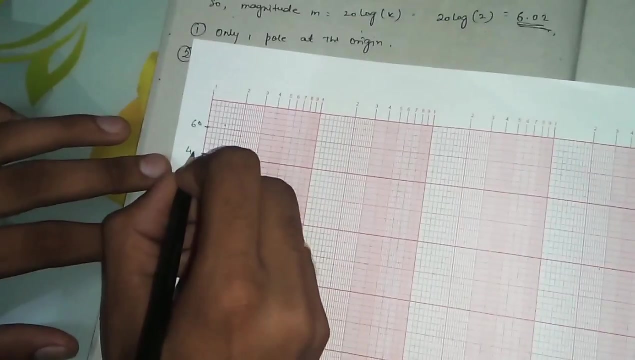 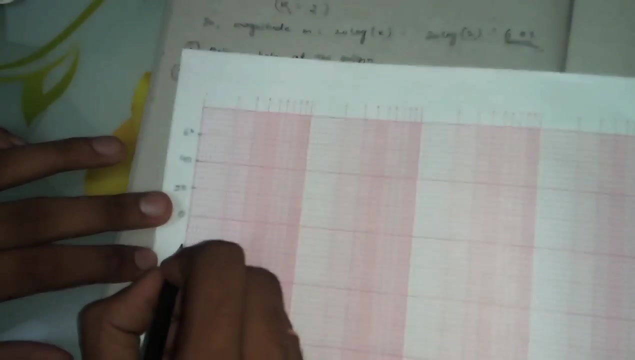 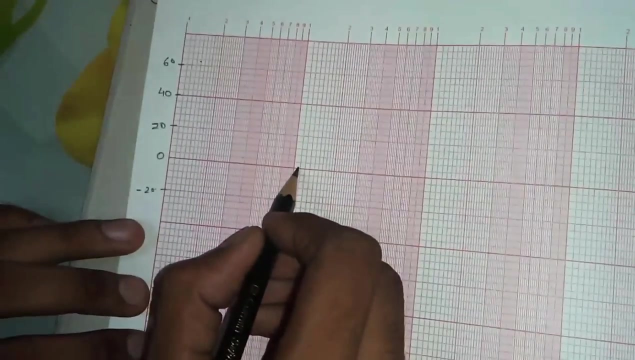 Now we will try to plot phase one. So we have two Omega values, 2 and 20.. So first we will plot the overview of it. So this is 60,, 40,, 20,, 0 and minus 20.. These are the magnitudes and this is my reference line and the phase angle starts from here, like 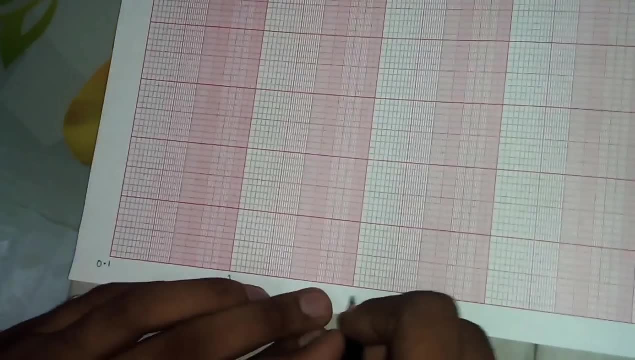 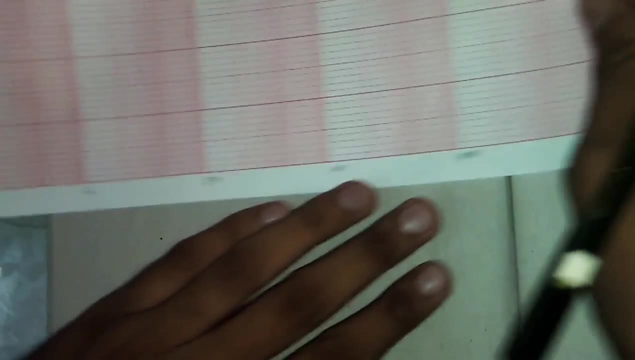 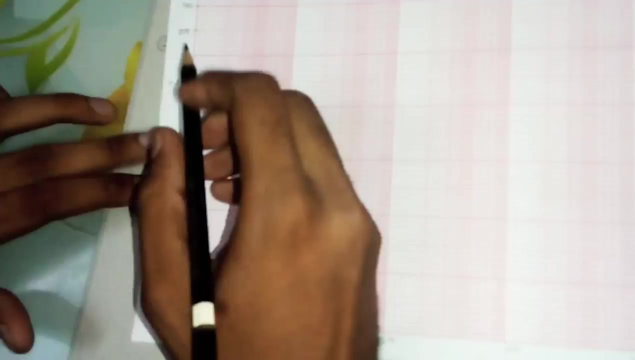 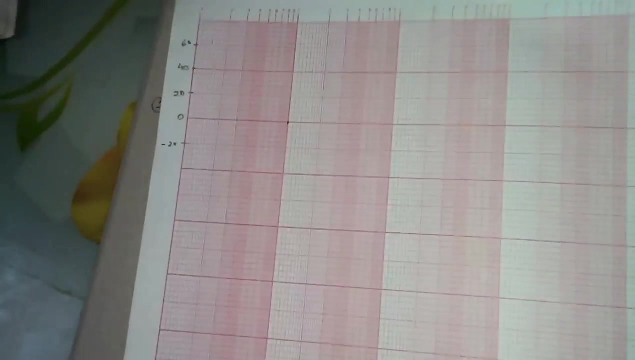 this. So this is 0.1, 1,, 10,, 100, 1000 and 10,000.. So first rule is we need to join all these points to the origin 1.. This we are doing just because of reference. 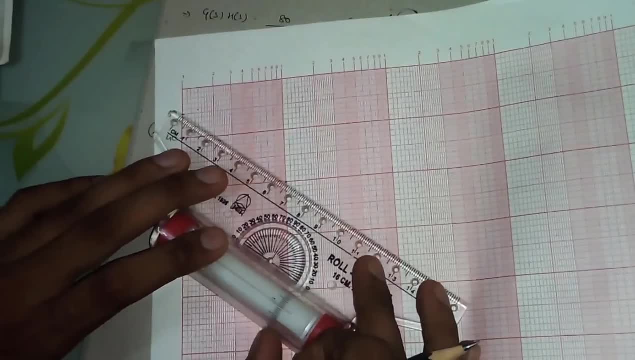 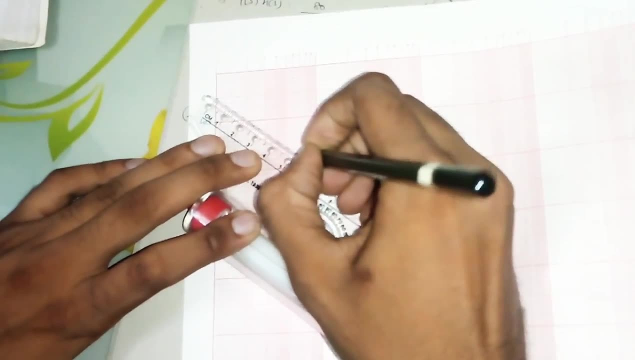 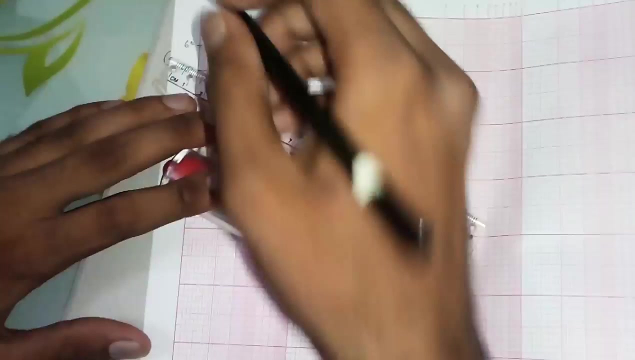 We will do this with the dotted line. So here we have the origin 1, and already we egged this. this is 0.1.. 0.1,, 0.1,, 0, 1000,, 1000 and 0.4.. 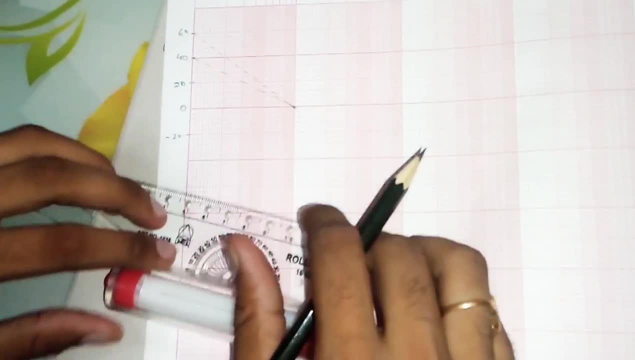 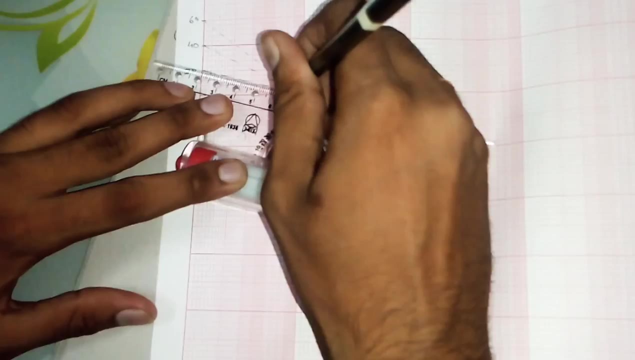 The next point is pure silence. So everything has been devoted for the duration as a spectrum. By the way, there is one more � benefactor, which is the Bridge Analyzerasa. So every point ishole. It's not a free control. 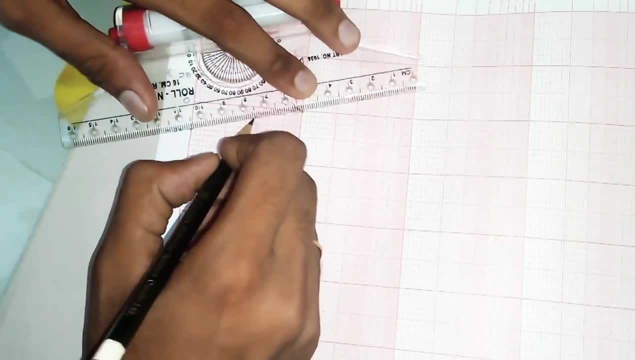 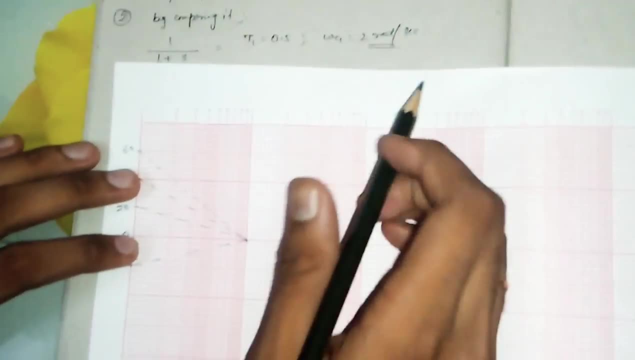 Okay, so now you breakdown every point and then changing position for the next, being neighbours stand. So every point has to be done till the origin zero. so it is done. now we'll check what is our k value, what is our magnitude. that is 6.02. 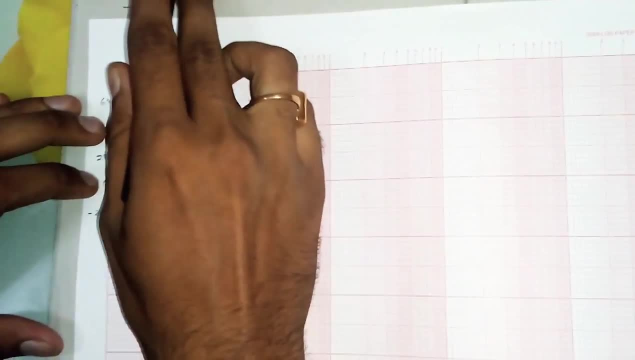 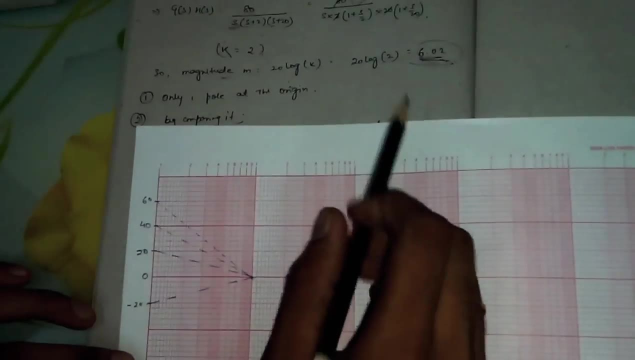 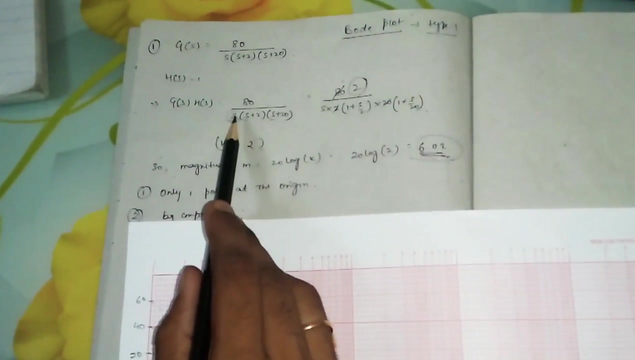 so, though it is a type 1 problem, we have got s. many of our youtube friends have done mistake here, like they have started plotting 6.02 directly from zero, but that is wrong, though we have s at origin, so we'll. we'll add 20 plus this like: 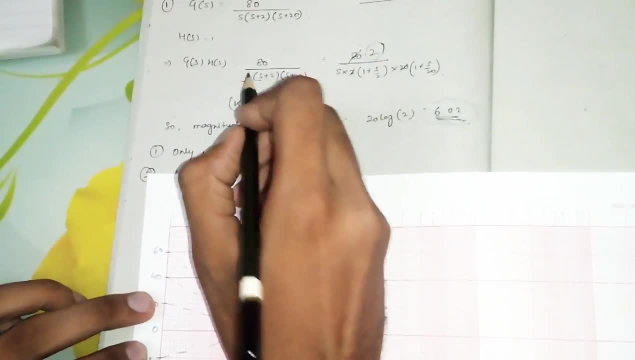 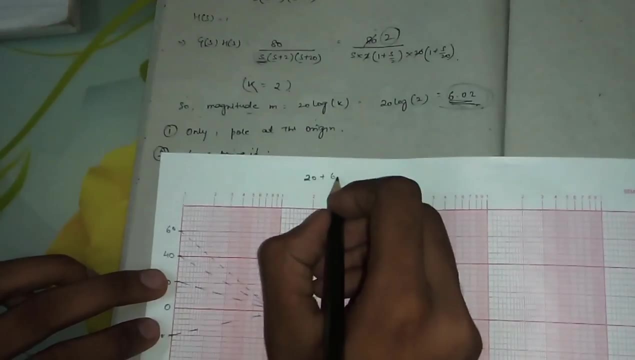 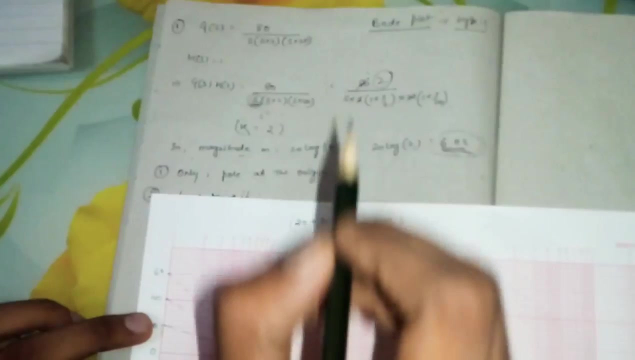 we have only one pole at the origin, so we have 20. we'll take 20 as a reference. plus this magnitude value, that is 6.02, is equal to 26.02 if we had this one s square, so we'll write 40 plus. 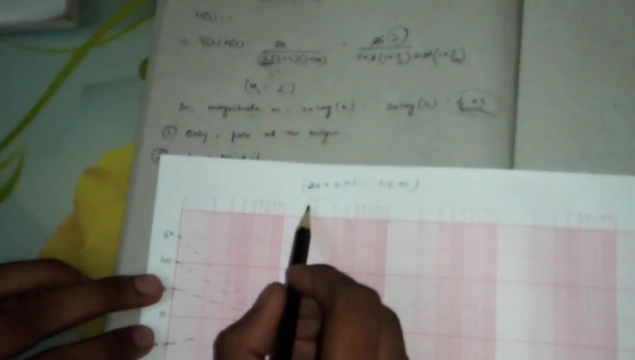 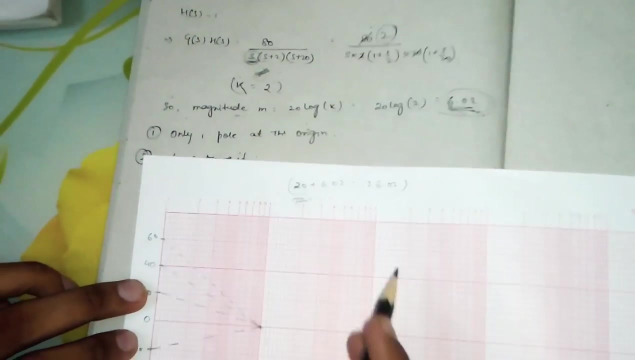 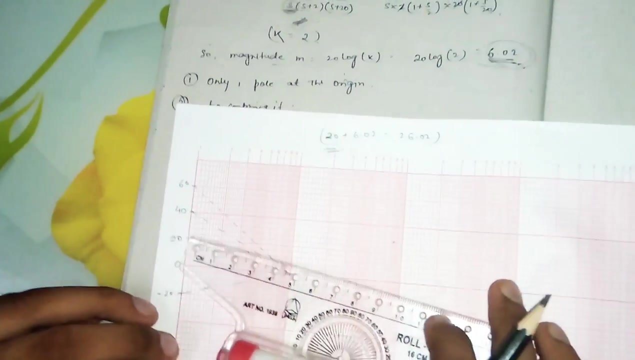 6.02, that is two poles at the origin. that's why we are taking 40, so here we have only one. so we'll use 20, 20 plus 6.02. this is our 20 log K line. so we'll plot in the graph. so value is 26.02. so each division, this small, small, each. 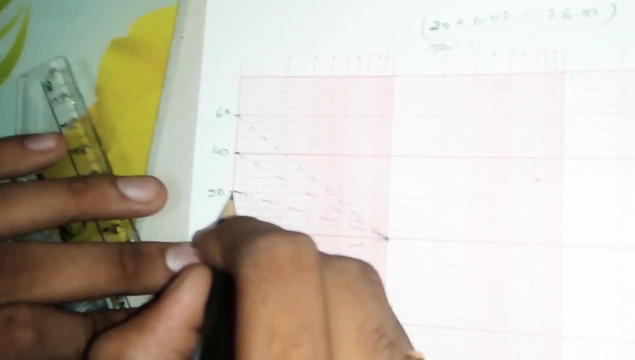 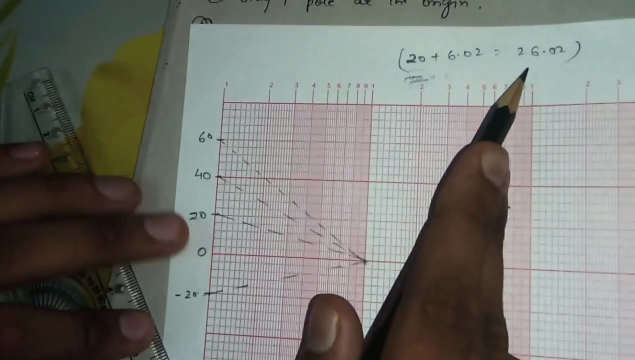 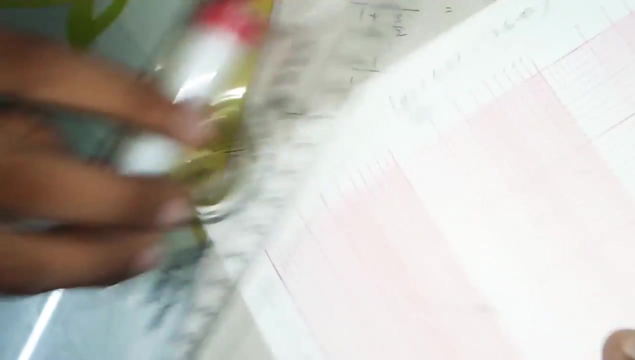 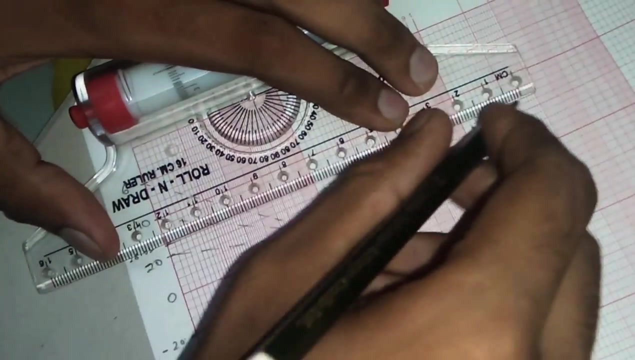 division is 4. this is 0, 4, 8, 12, 16, 20. so we have got 26 point 0, 2. this will be here: 26 point 0, 2. we'll draw this with light line. this is our reference line. 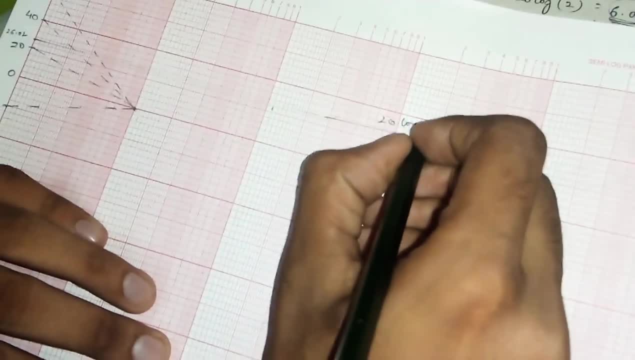 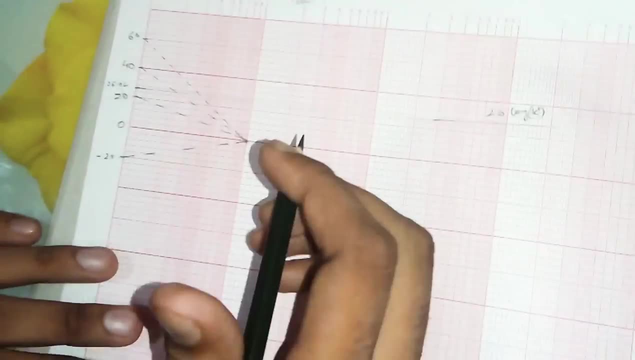 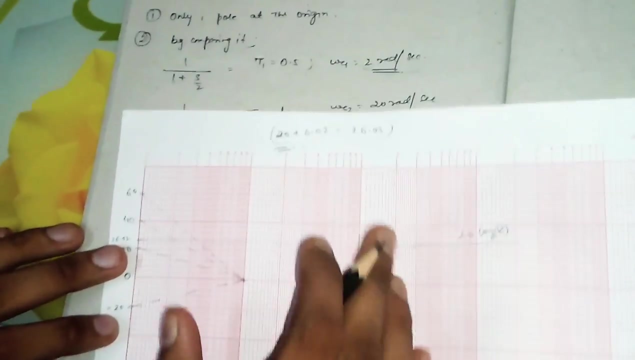 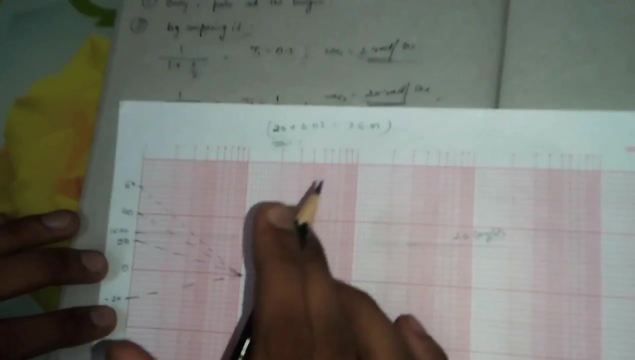 this is Now it is done. Now we will start our plotting. So first is 2 radians per second. Everything which we have to draw, like we have, this is one pole at the origin. so we will draw a slope of 20 decibel per decade. So we will draw 20 decibel per decade If it is s square, like. 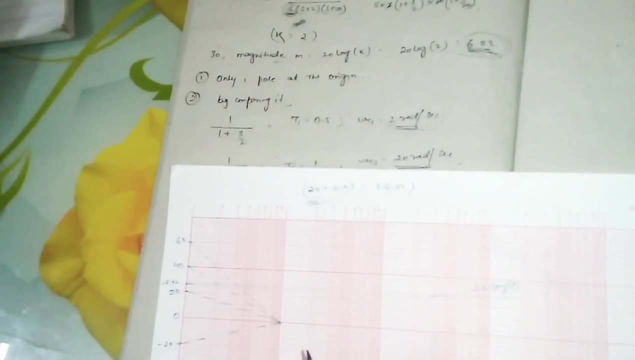 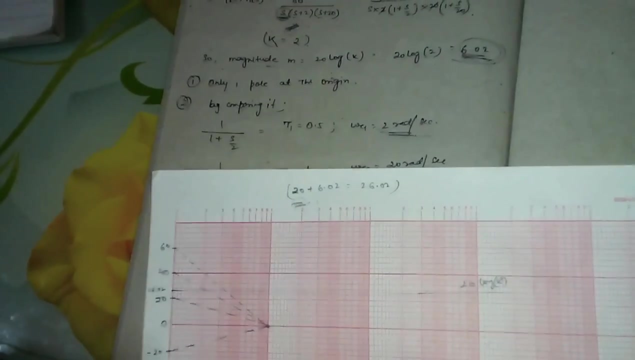 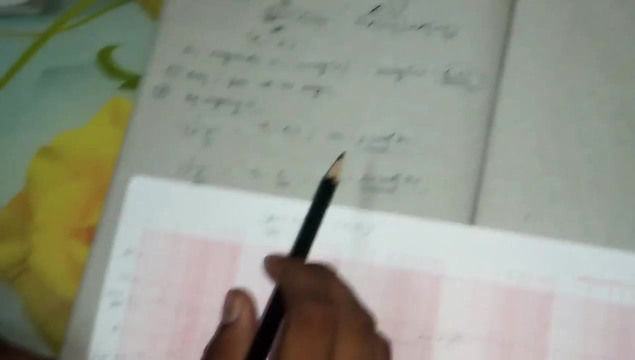 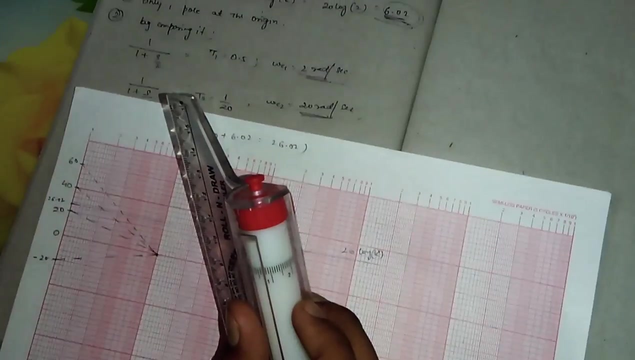 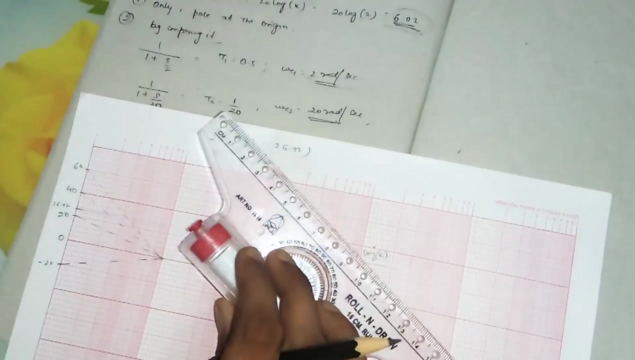 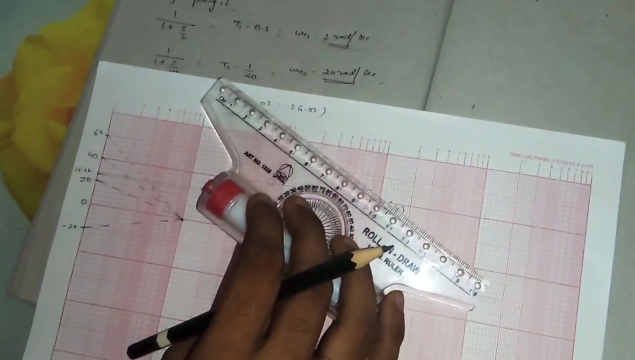 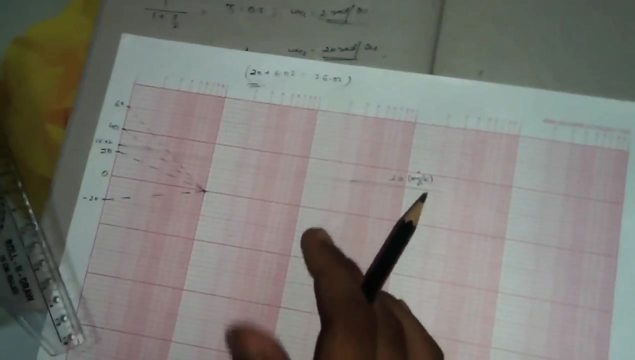 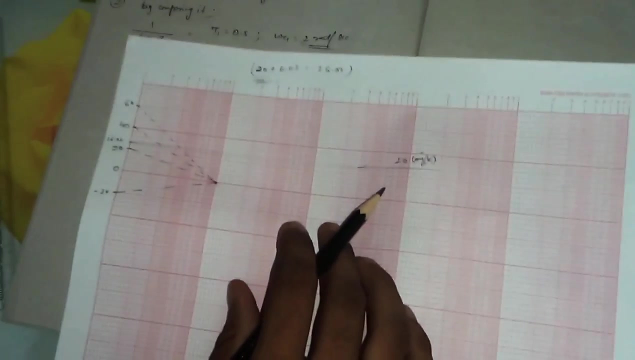 type 2, then we would have taken 40 decibel per decade. So here we have only one pole at the origin, so we will draw 20 decibel per decade. 26 to this will be a 27 per decade till the, till which one we have to go till 2 till 2 we. 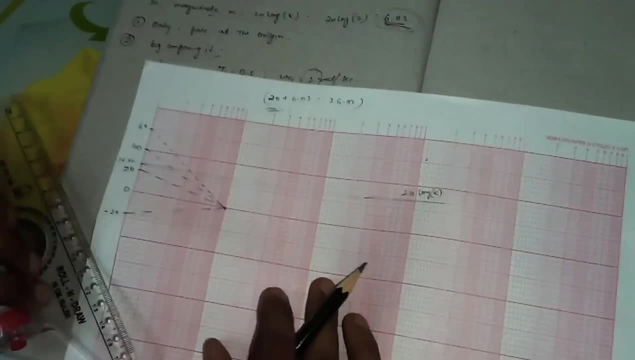 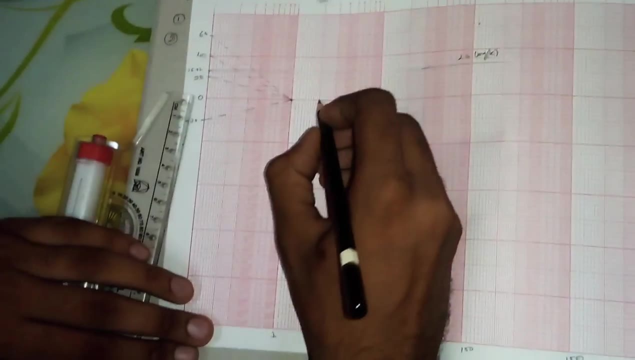 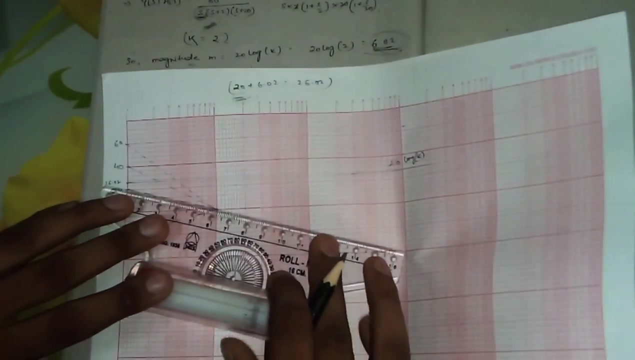 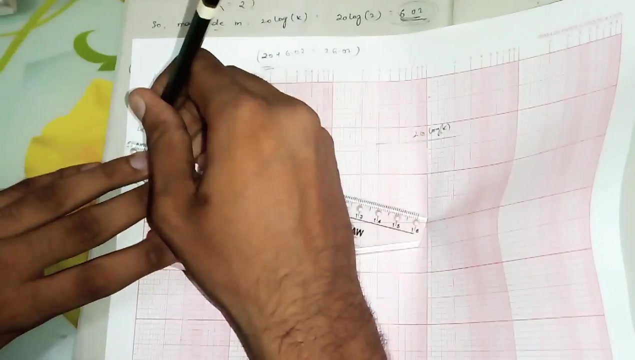 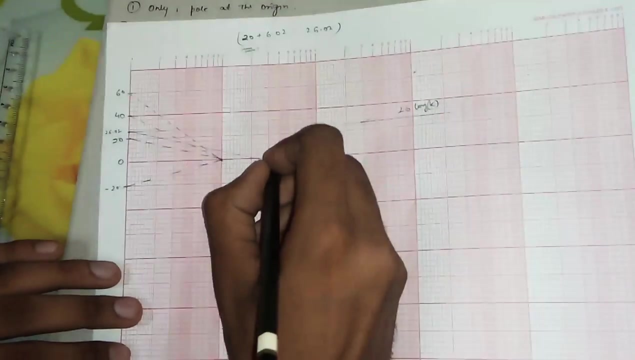 have to go. So, ok, from here we will start till 2.. 2 is this, one means this line is 2.. Ok, fine, We will take the slope of 20 from here. So to: this is our omega c1, and this is minus 27.. 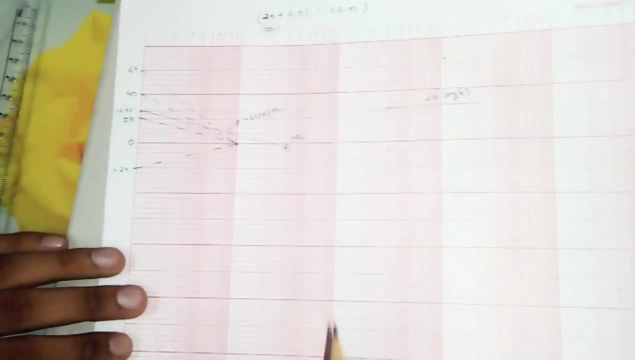 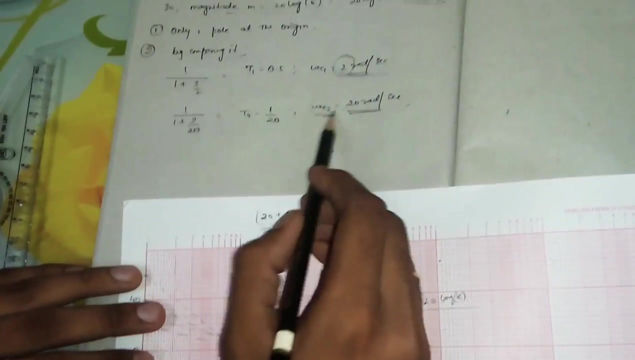 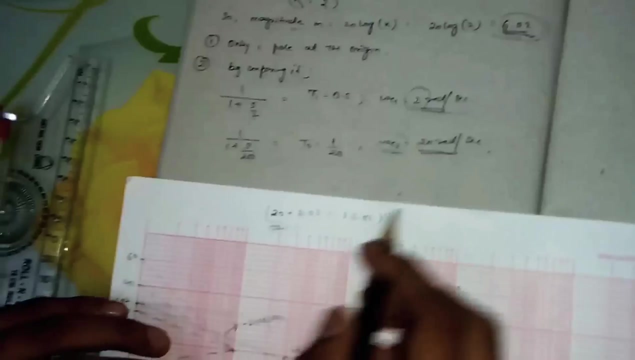 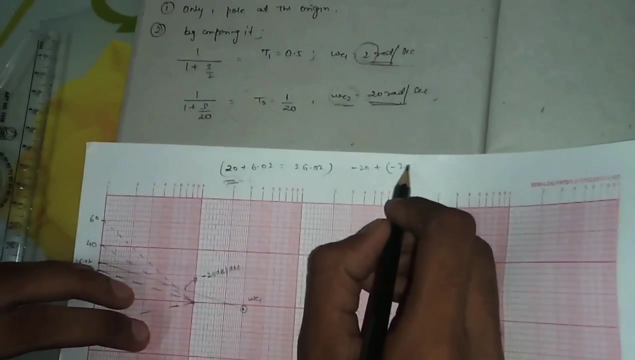 20 dB per decade. This is our omega c1. Next we have to go to omega c2.. That is 20 radians per second, But both are pole. So what we will do here, We will do addition. So minus 20 per decade, plus of minus 20 per decade, That is minus 40 dB per decade. So this is. 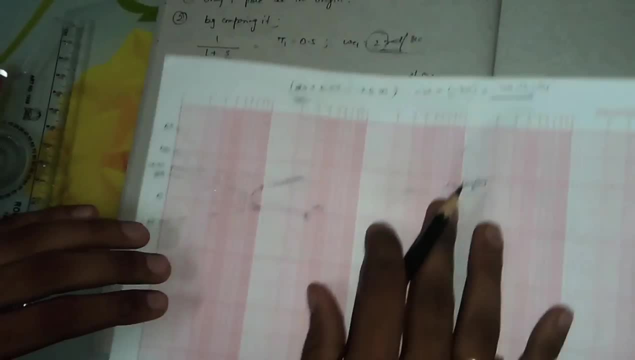 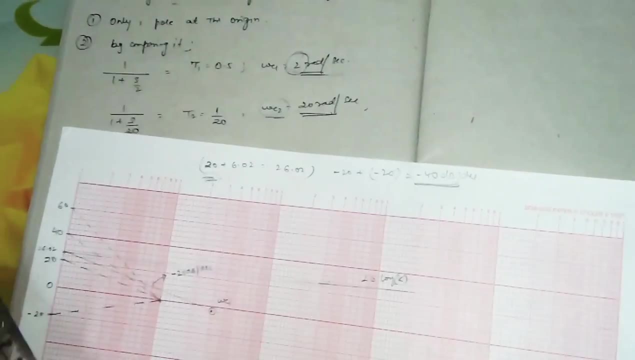 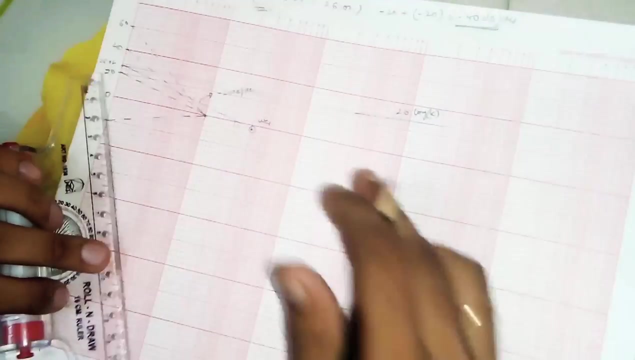 minus 40 per decade. So with the slope of minus 40 per dB plus decade, We will draw a line till 20.. 20 is which one? This one is our 20.. This one was our 2. So till 20. 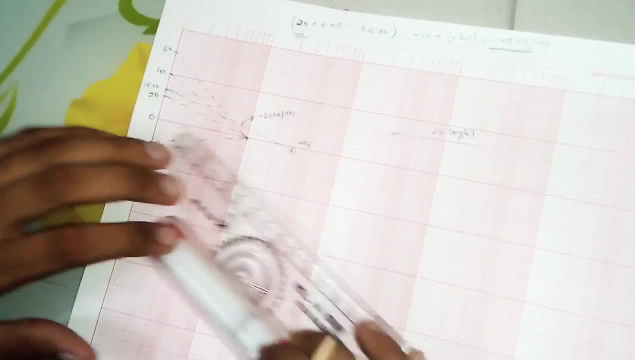 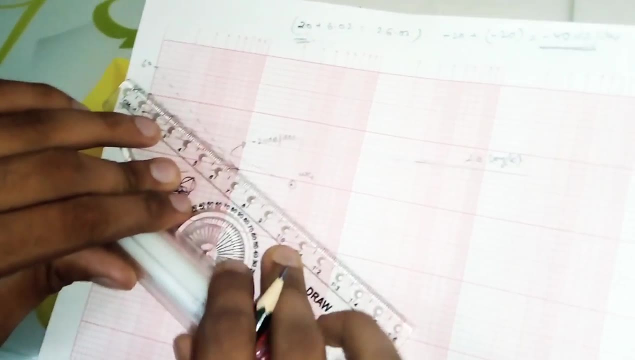 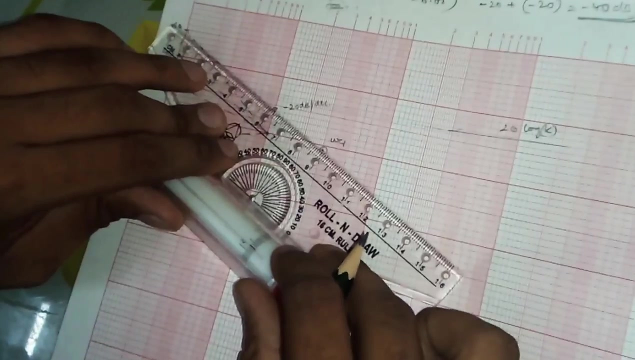 we will do draw a line, the slope of 40. So this is our 40 slope. We will take up to minus 20 for this line. So we will start towards our 40 slope and we, now we have come here, 20, we have to go in this. We have to go in millimeter square. the fixate Forum. Now you. see what is standing: 10, 4 feet. Here it goes Now where I have done this t. this line color is different, it is thin. in these two It cannot be even so many. Okay, point 5, 2, the point which I am going to solve it. we can do it from here, This line line. here again I will. draw a number. Now I have to go back 2 by RT away from the carreer. At this point we are going to press this ladder all the way to the left, and what case will happen? to what east? Now let us go, guys. which lane has led to the right side? Now, if 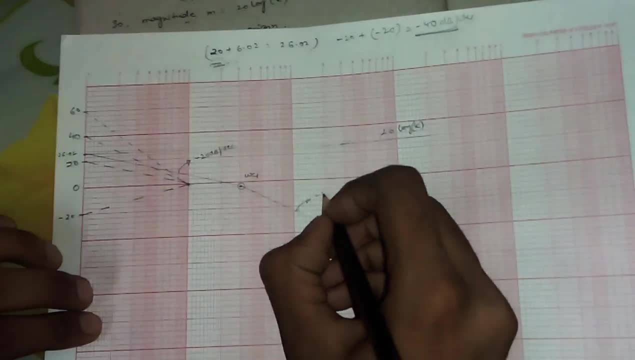 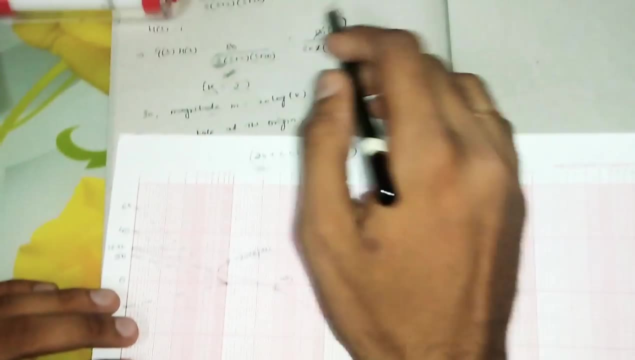 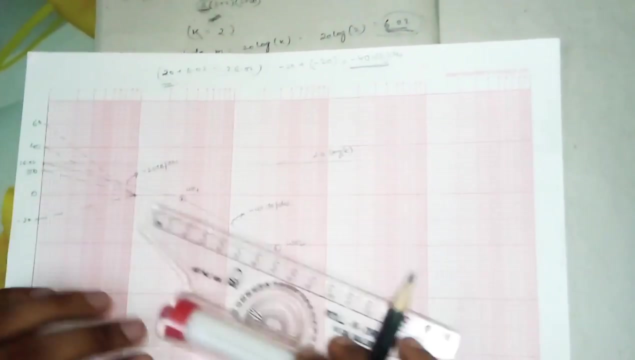 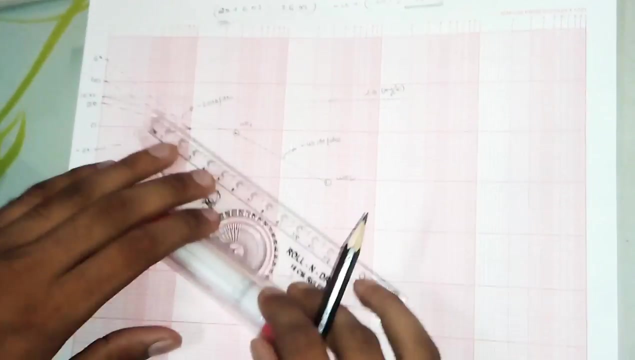 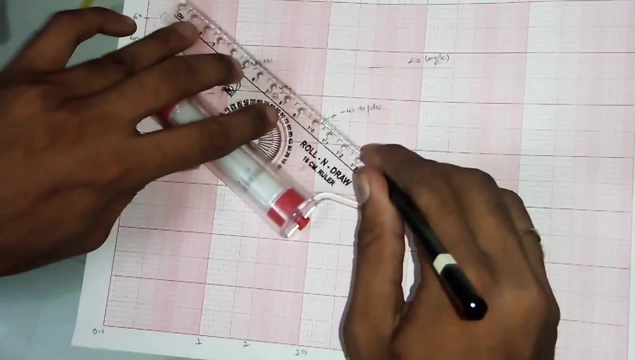 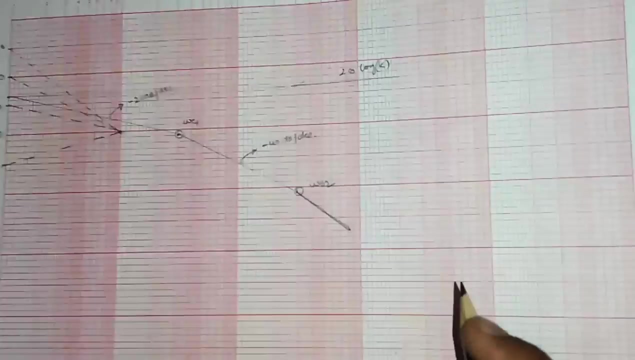 c2 with a slope of minus 40 DB per deck, and though we don't have anything other poles, so we'll draw till infinity so that this can be of any slope will take 60. draw a small line, it is not so you, it is not so useful. so that's how the 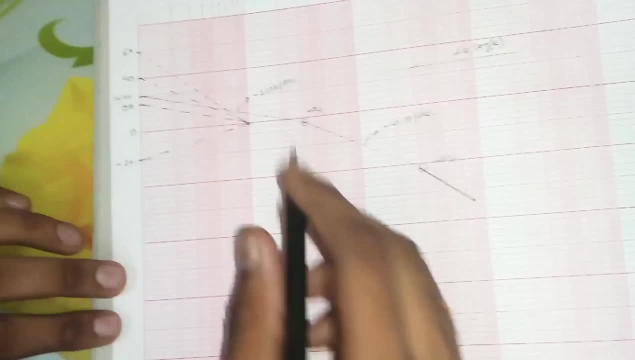 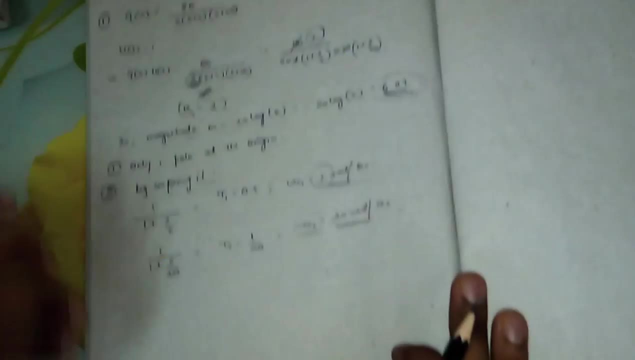 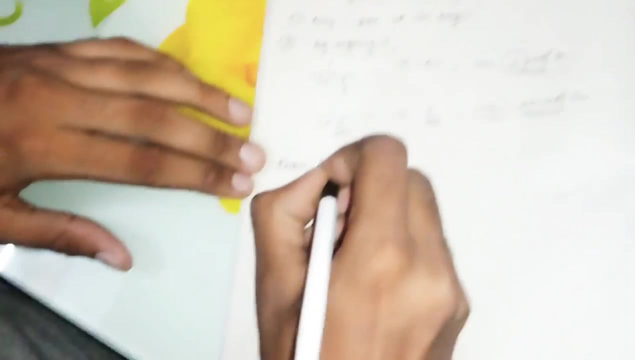 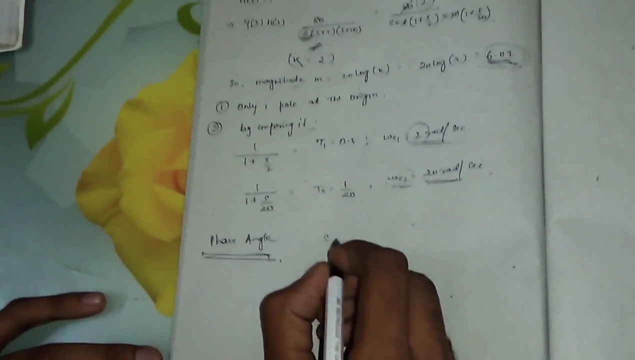 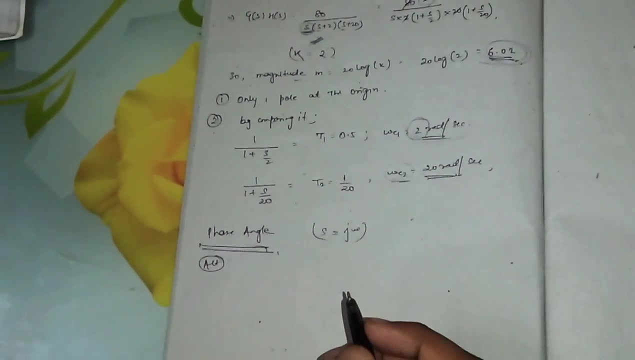 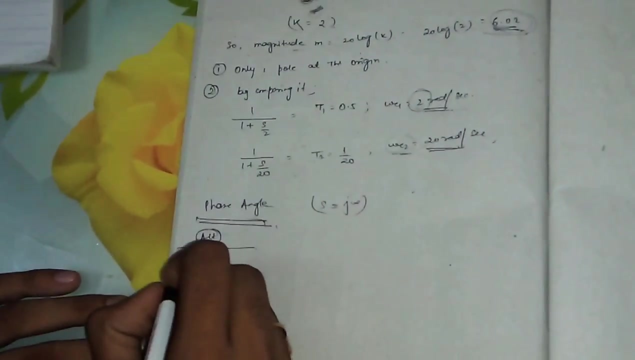 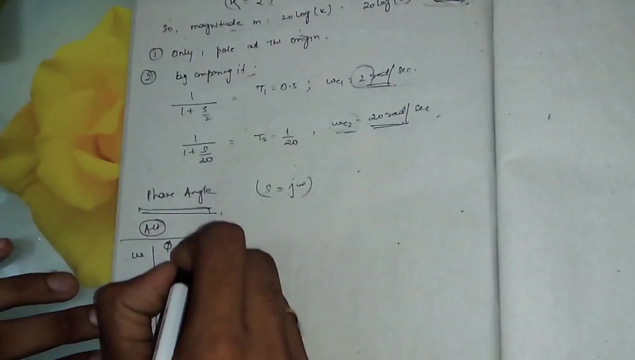 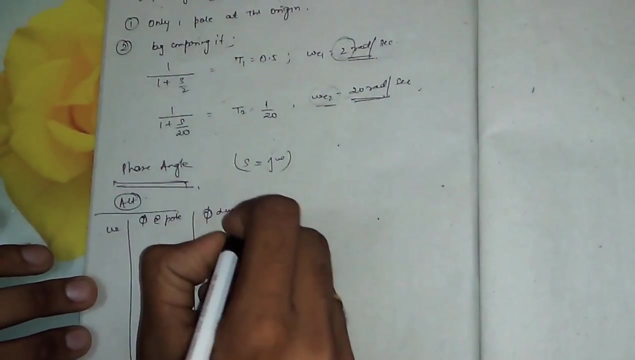 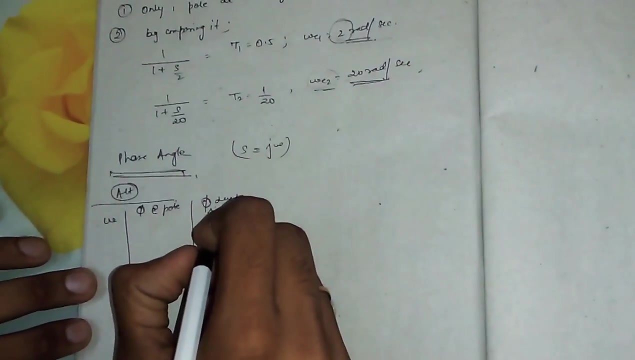 magnitude plot got gets over. now we'll go for the phase angle plot. phase angle, so simply, without putting s, is equal to j, Omega. we can go with another alternative, which is very easy, so we can see that we'll plot a table. we plot a table that is Omega Phi at pole Phi, due to simple pole, where t1 is 0.5, here phi. 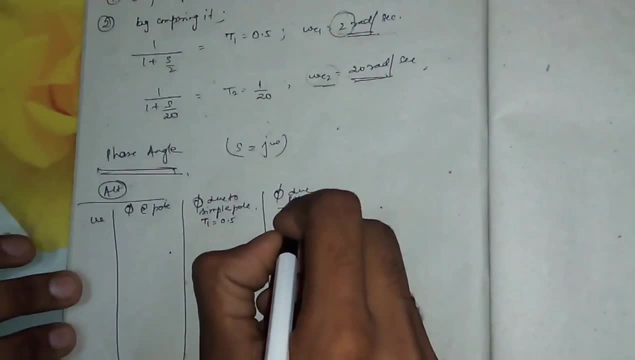 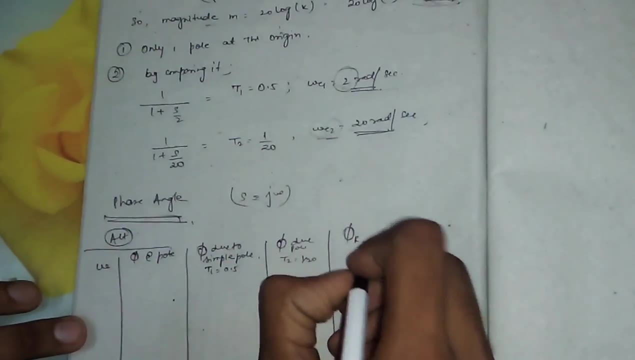 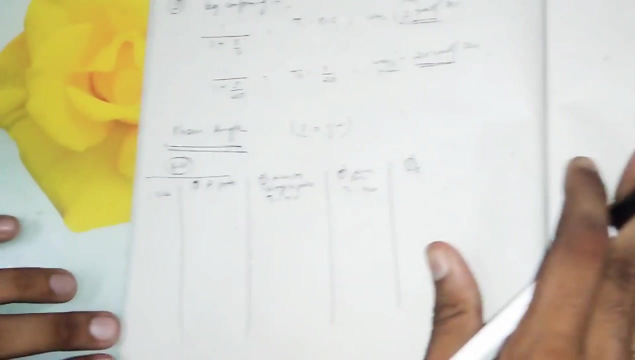 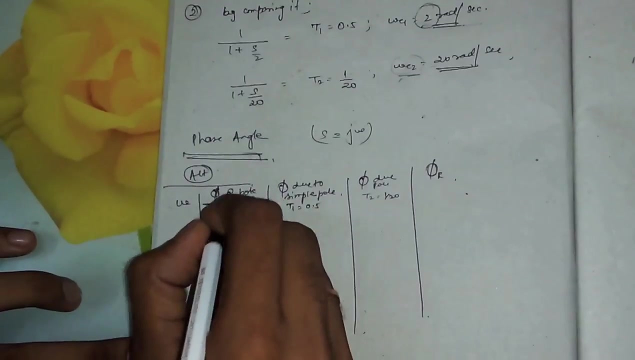 due to simple pull. again, 52 is equal to 1 by 20 and 5 are. so we'll try to cover this. two points in our table and the most important thing is 5 at the origin. this is at the origin, so we have one pole at the origin, so we'll take minus 90. it would have taken. 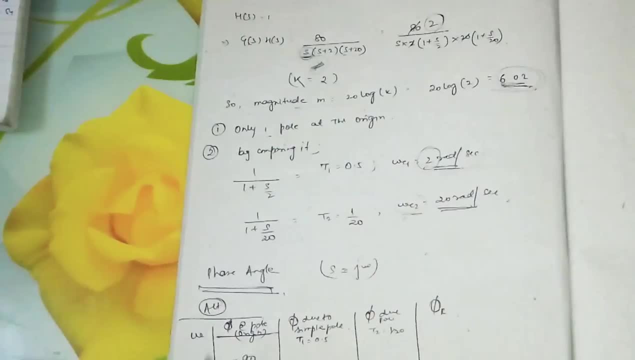 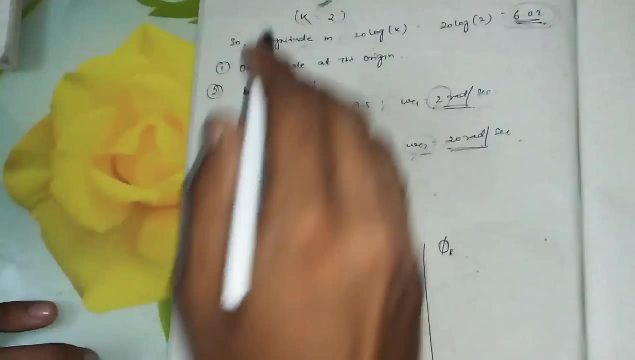 it would have a square like two poles at the origin. that would be minus 180. so here we have only one pole at the origin, so we are taking minus 90. if we have two poles at the origin, then what we have done and then what should we do? minus 90. 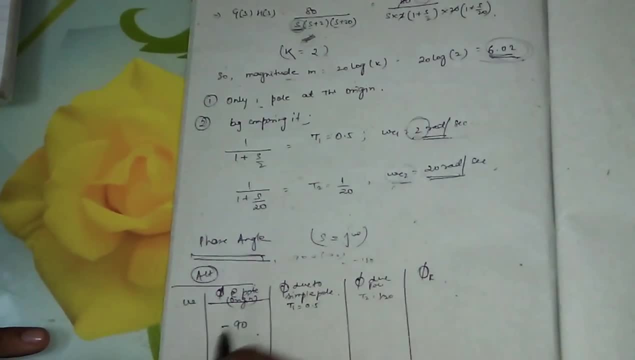 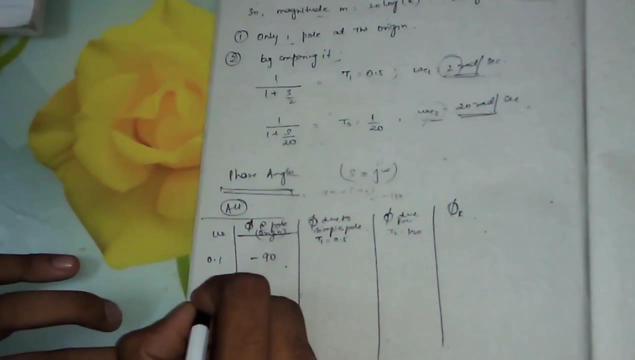 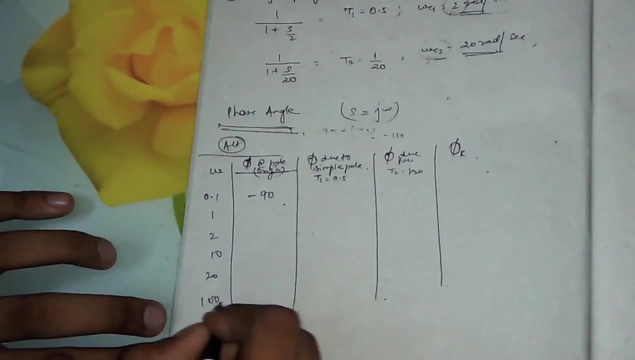 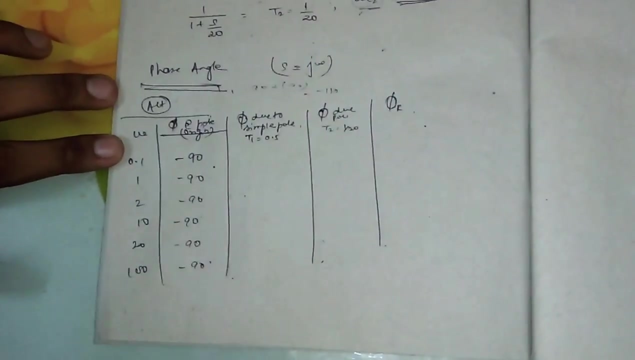 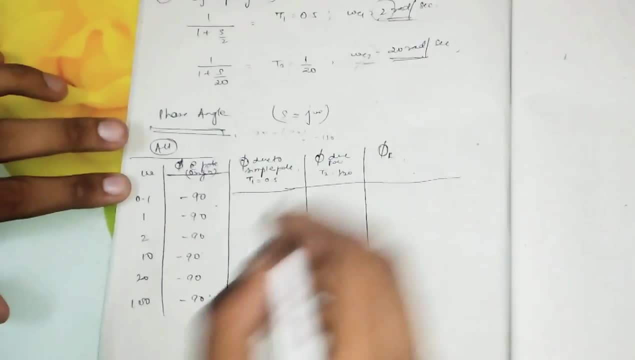 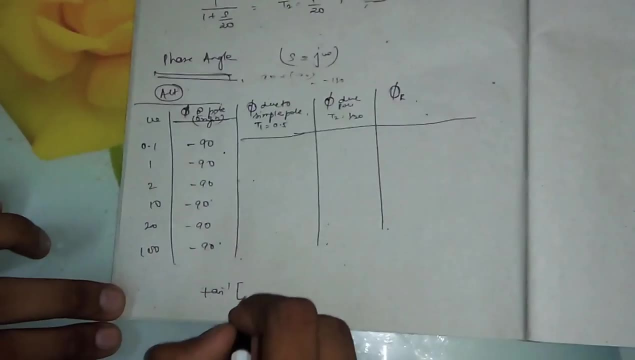 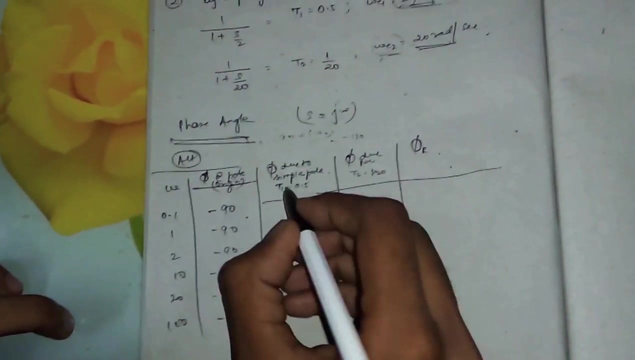 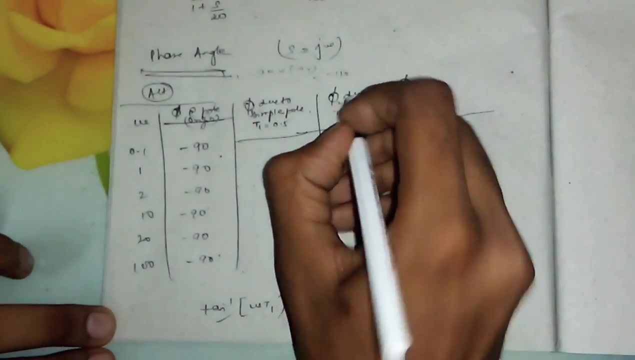 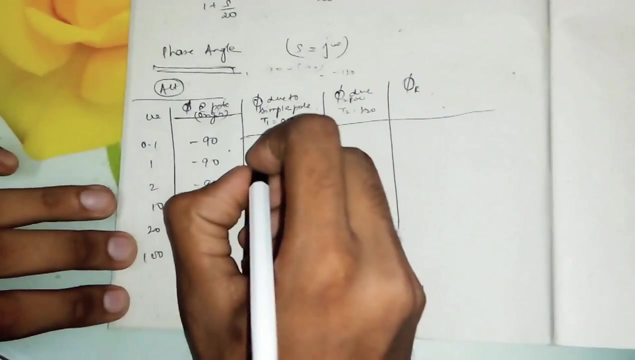 formula here is to calculate t1. the formula which we are using is tan inverse of Omega t1 and tan inverse of Omega t2 to calculate this part. to calculate phi 1 is this one? to calculate phi 2: is this one? so I have listed my values. I will be writing it immediately. first one is minus. 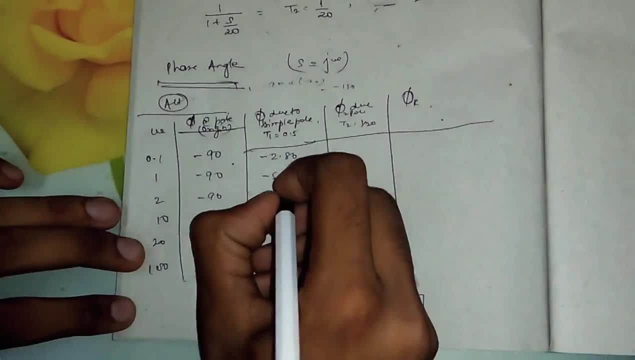 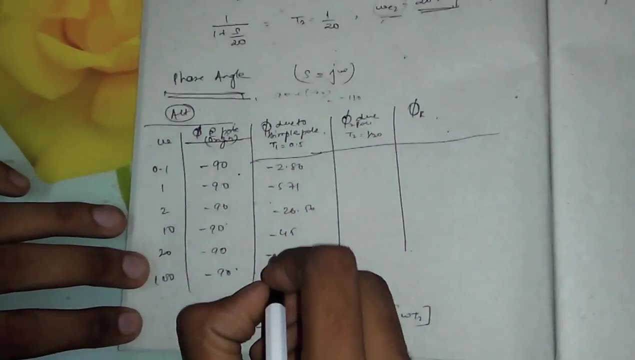 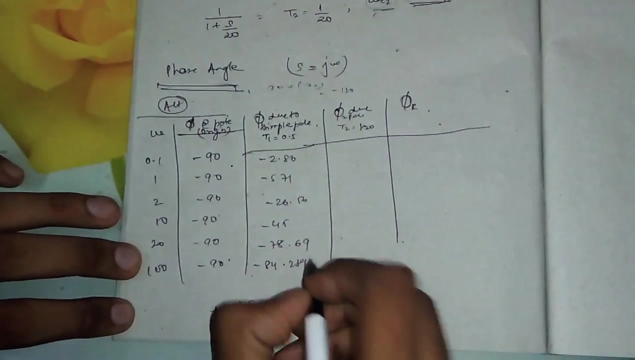 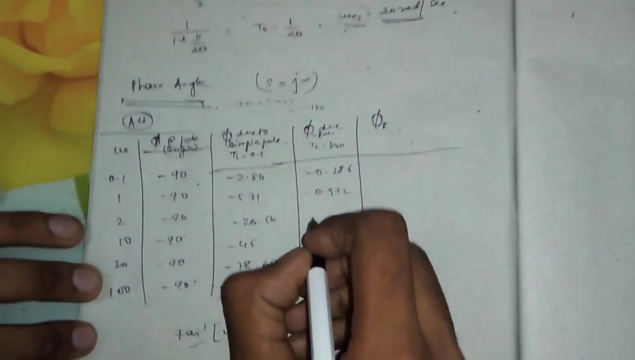 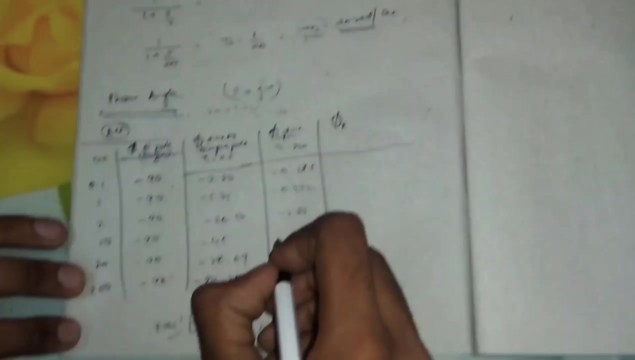 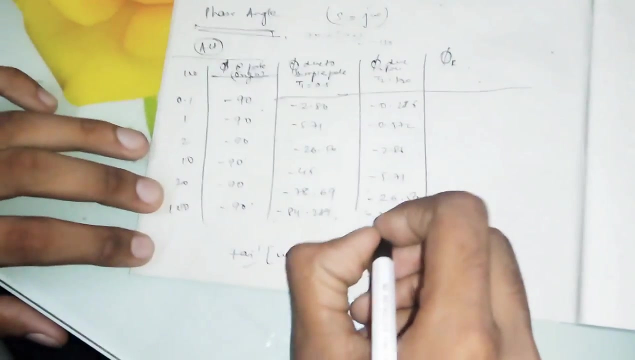 two point eight. six minus five point seven. one minus twenty six point five. six minus forty five minus seventy eight point six nine minus 84.289 minus 0.286 minus 0.57 to minus two point 86. next one is minus five point seven. one minus twenty six point five. six minus seventy eight point. 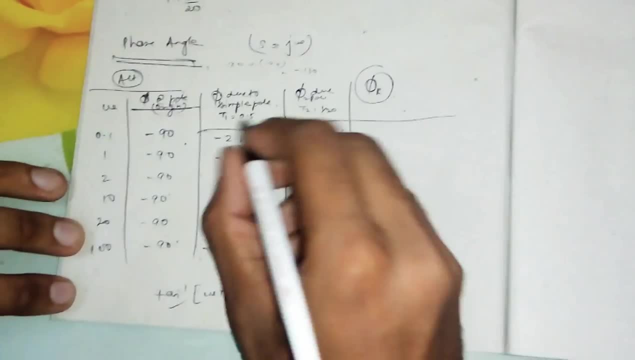 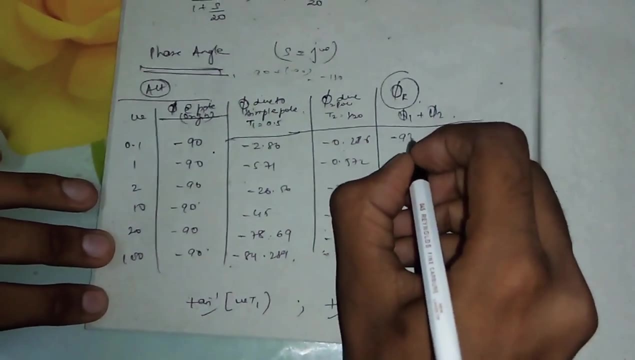 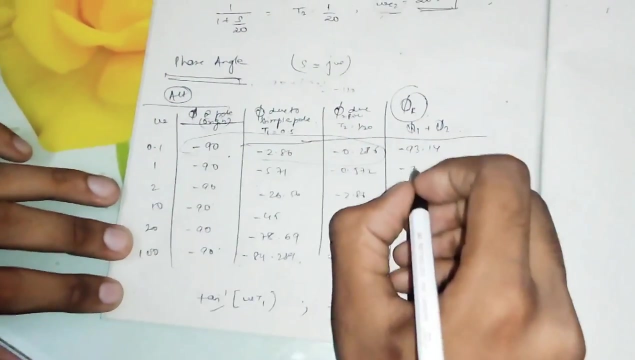 six nine. this are is the sum of first and second: 5, 1 plus 5, 2. this is fire minus 93 point. 1. 4 minus will do the addition of this total. total addition is here. will do here and then minus 96 point to. 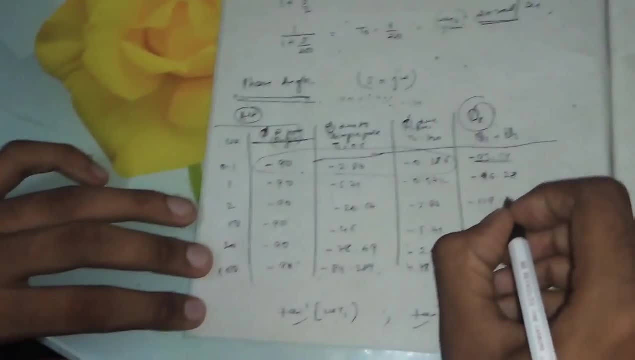 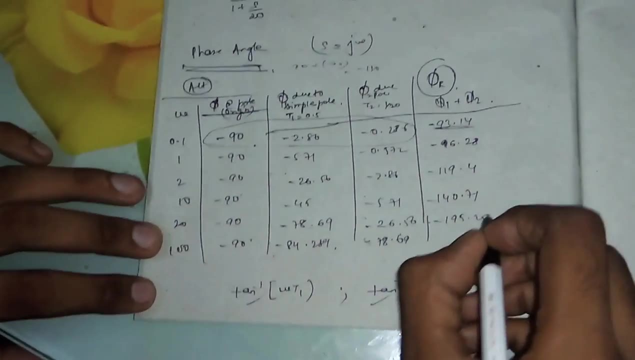 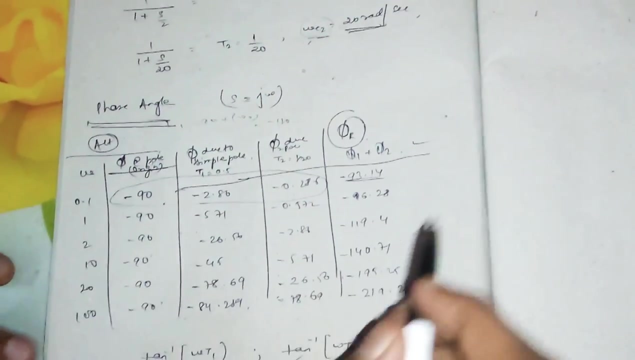 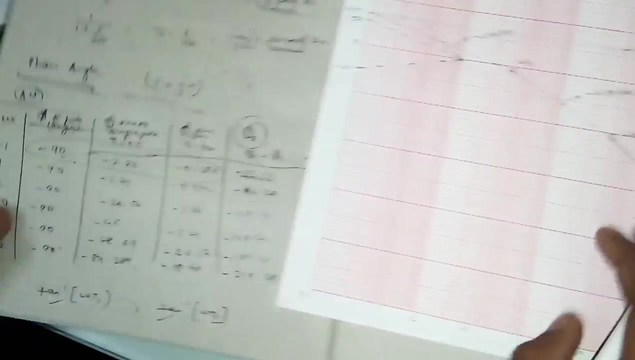 it minus 119 point 4 minus 140 point 7, 1 minus 195 point 2, 5 minus 219 point to it. so it is a phase angle plot. go and get got ready this plot in our graph. so here the origin will be 90 degree. so we'll start plotting it without wasting. 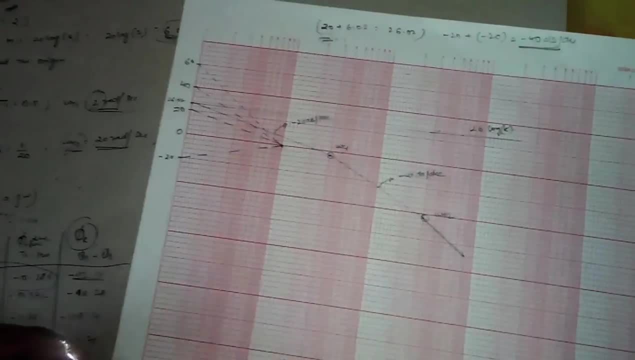 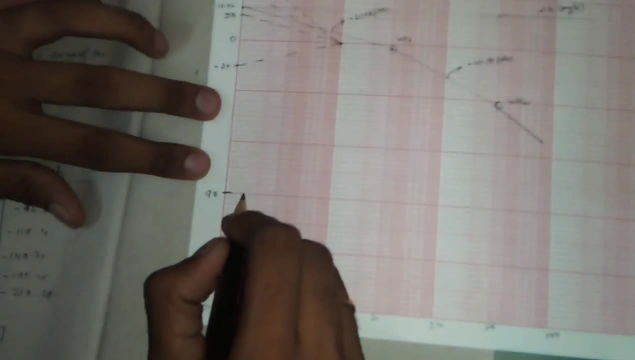 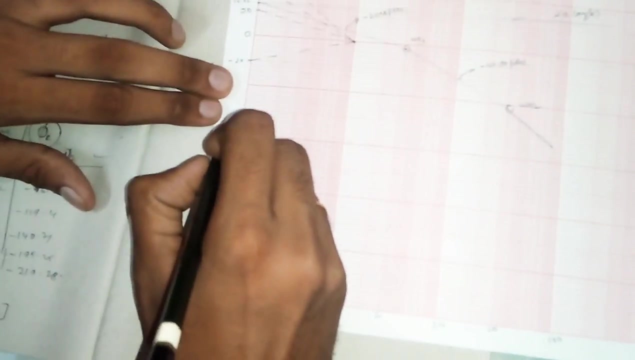 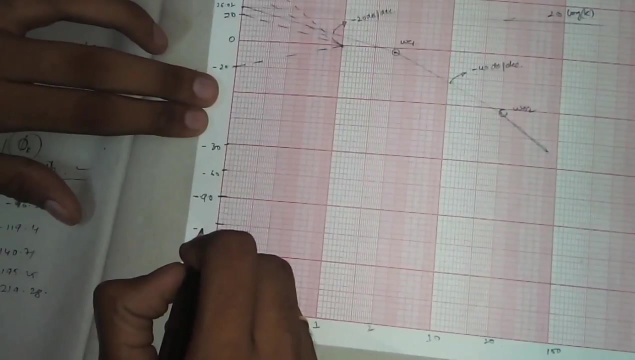 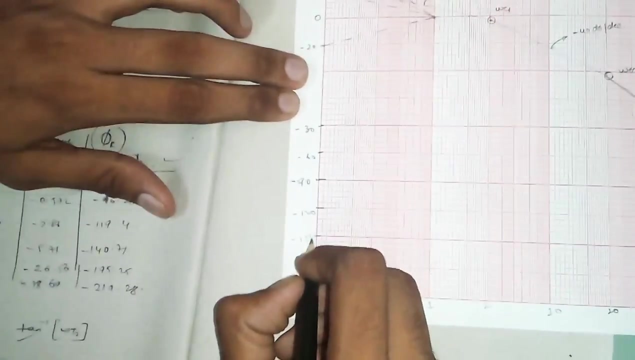 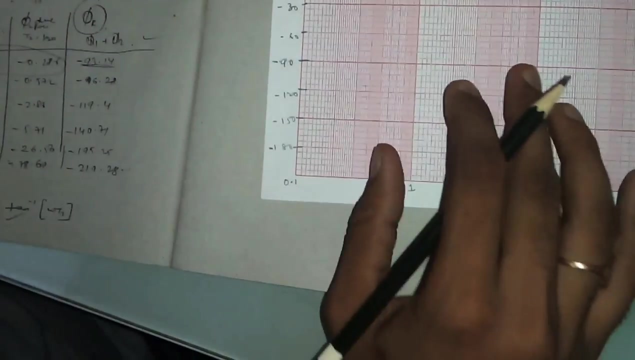 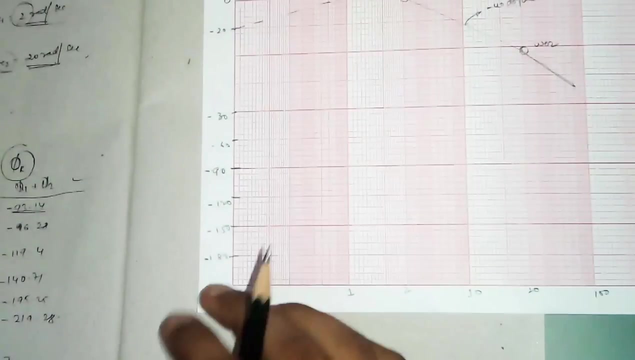 much time, so we'll take a. origin is 90, 9-90, our one will be minus 60 minus 30, and down part is minus minus 90, 120, 150, 180 in account of 30s will plot. so first one will plot at point 1, at at. 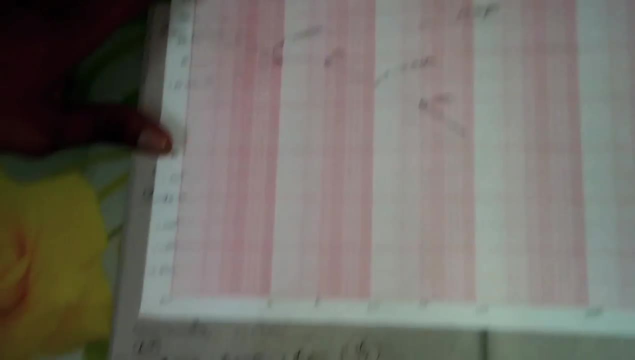 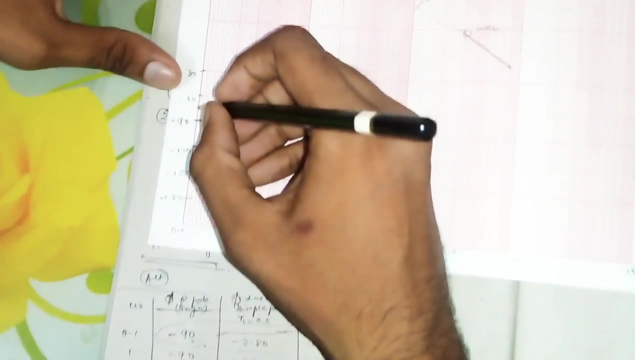 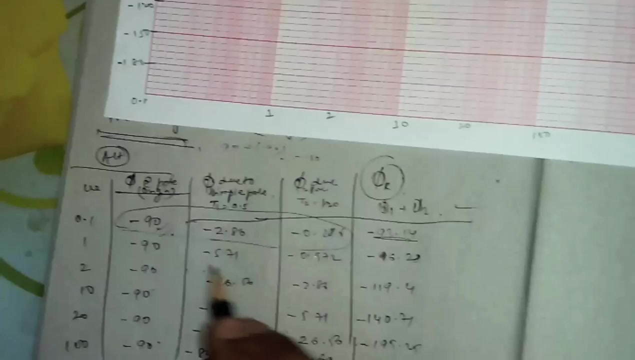 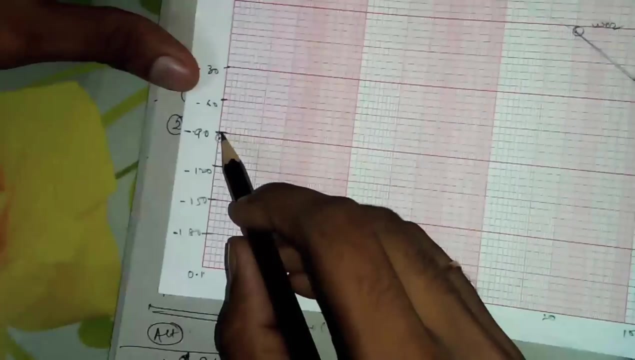 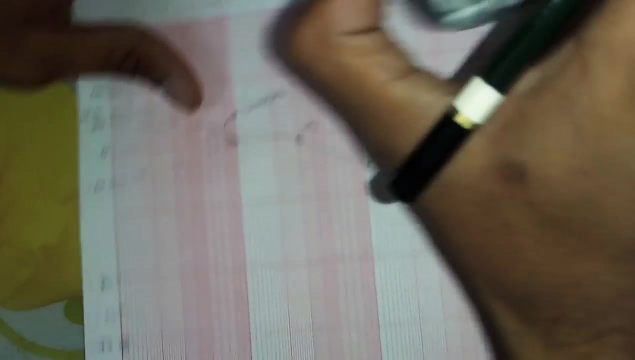 point 1: we got ninety three. point one, four. point one: we got ninety three, point one, four. that is from here first, first is this one, then comes minus 96 at 1, 96. this is 90: 1, 2, 3, 4, 5, 5 plots. so each plots will be: 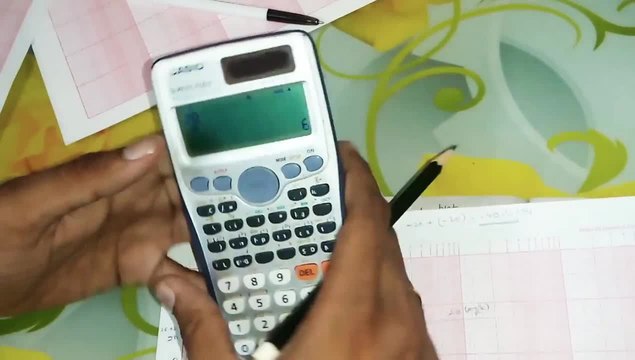 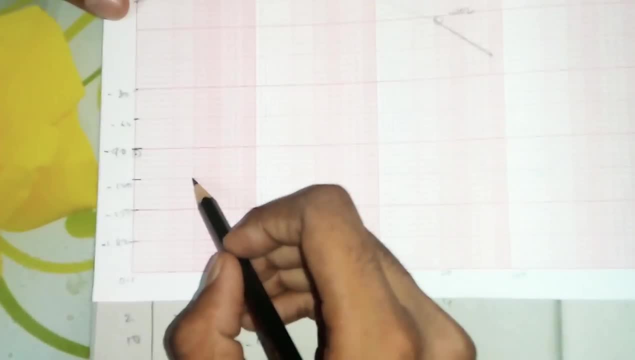 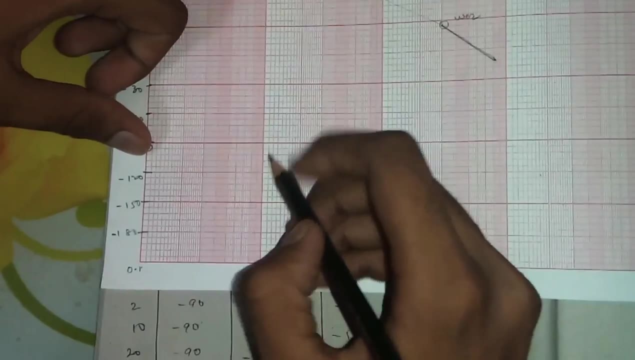 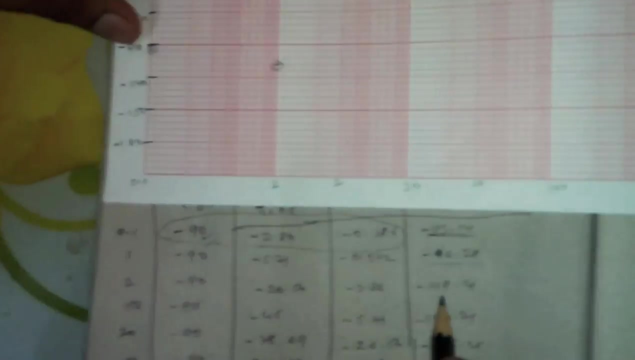 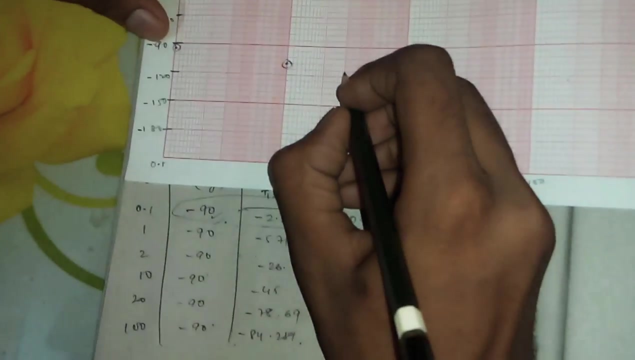 30 divided by 5, 6 of 6, so 96 will be somewhere at 1, 4, 6. this this will be 96 point to 8. then minus 119, point 4 at 2, 119 will be somewhere here then.